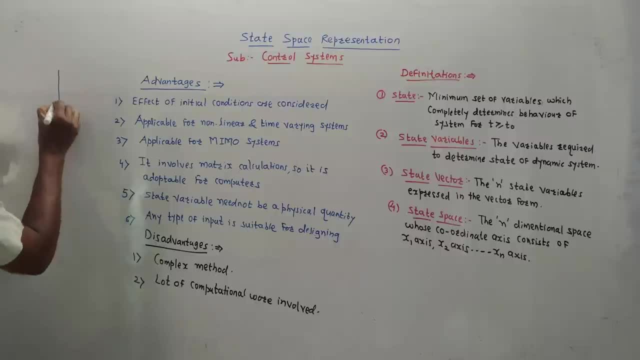 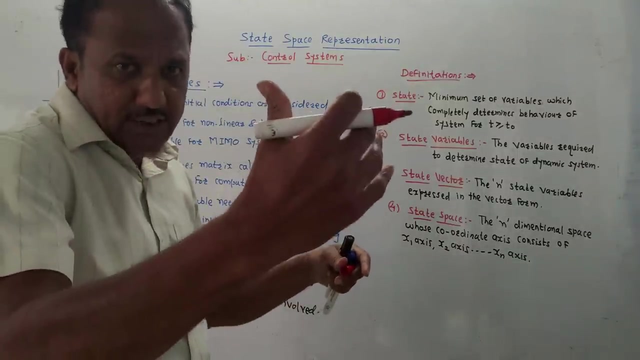 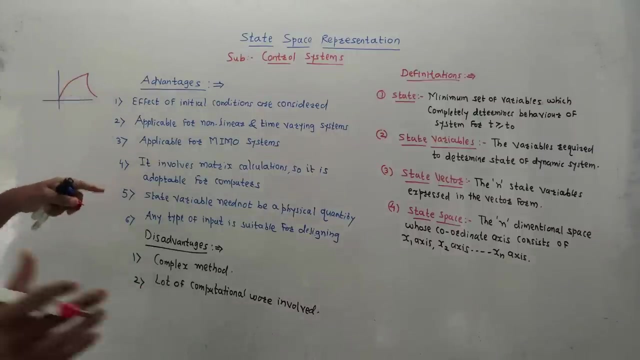 Now look, if you consider one capacitor, ideally the charging of capacitor starts from zero, like this. We know that it's exponential charging. Discharging is also exponential. Look, any capacitor starts charging from zero, So there are no initial conditions. But there is one capacitor which is not fully discharged and someone tried to use that capacitor. 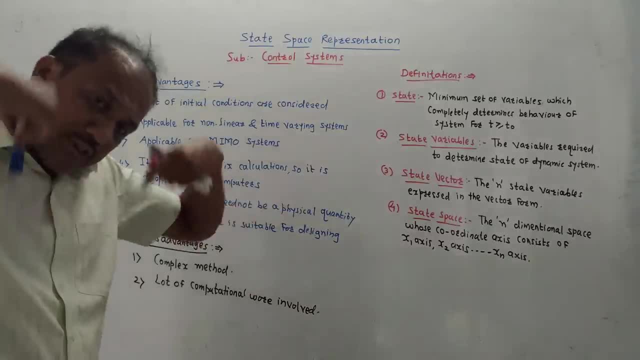 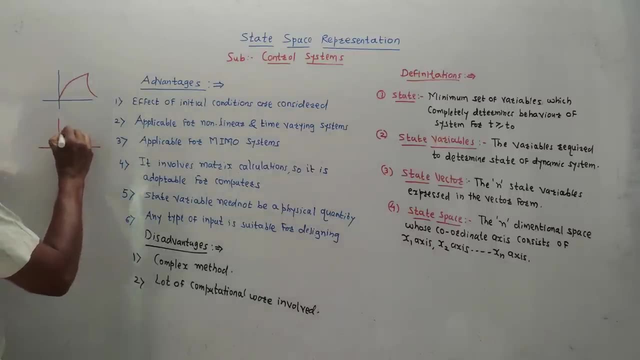 It means it is not fully discharged. If it is fully discharged, then it will start charging from zero again. If it is not fully discharged and someone started using the capacitor, then charging will not start from zero. It will start from some other value. This is called as initial condition, So this is initial condition for the capacitor. 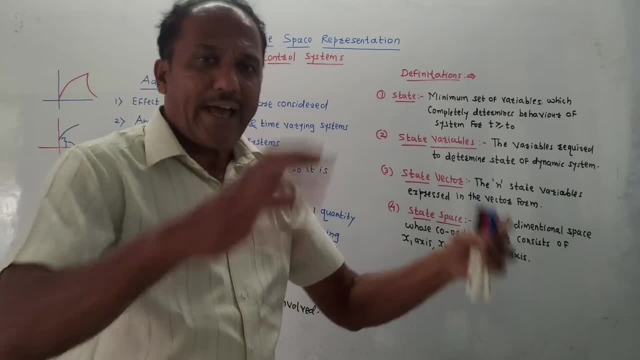 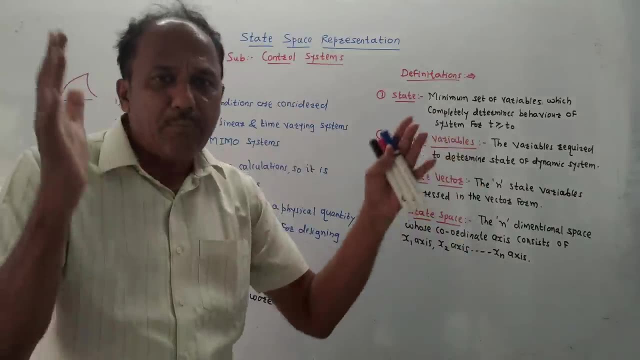 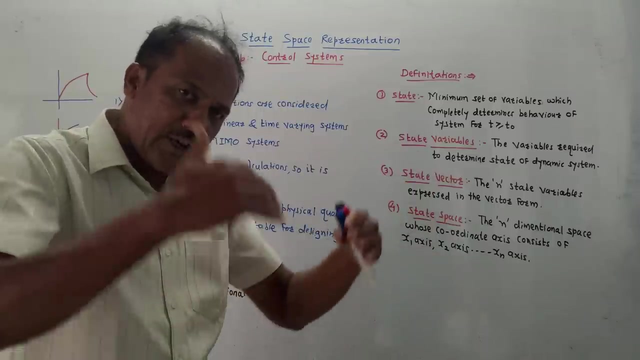 Now, if you want to calculate the output across any capacitor, you need to consider this initial condition. This is called as state of that particular system. So state means the condition from where you start. That also you need to take into consideration. This is called the state of a system. This is a broad overview that I have told you. 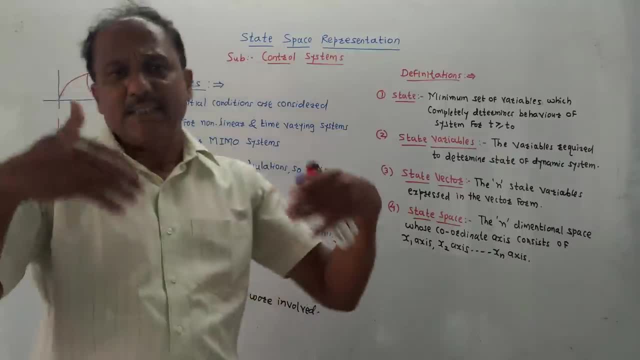 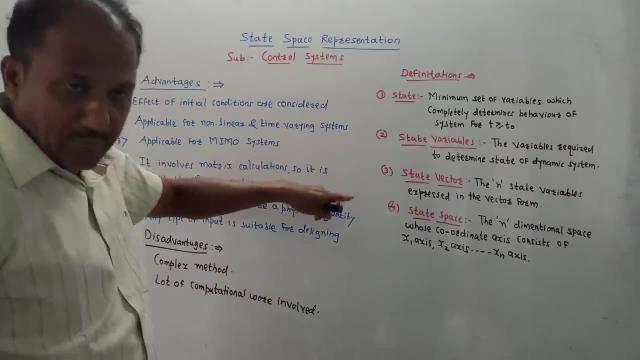 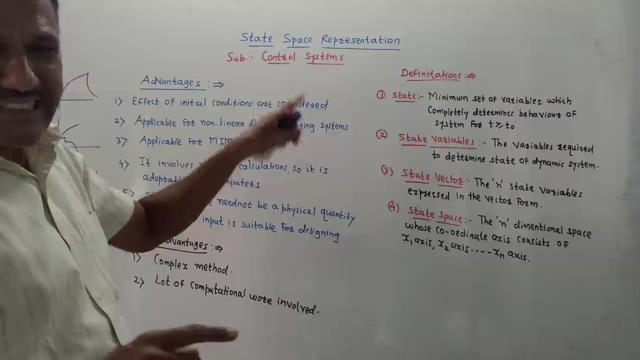 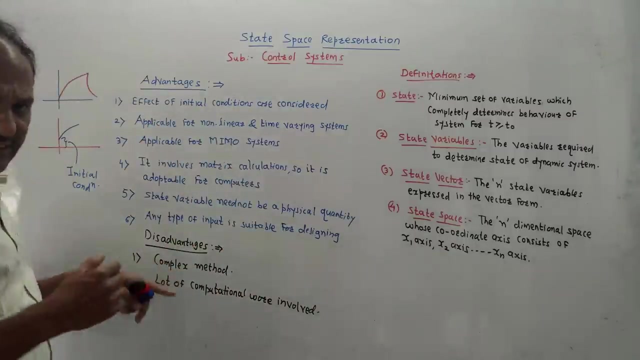 Now, whatever methods we used before this analysis, those are called as conventional control system methods. In this unit, ie in the state-space representation unit, we will be using some different techniques, which are called state-space analysis techniques. Now, what are the advantages? Sometimes, from the exact point of view, advantages as well as disadvantages are asked. 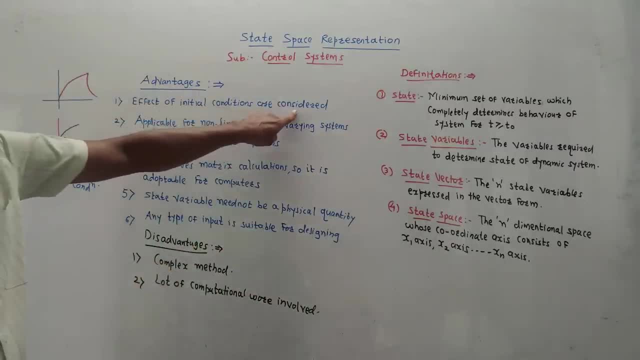 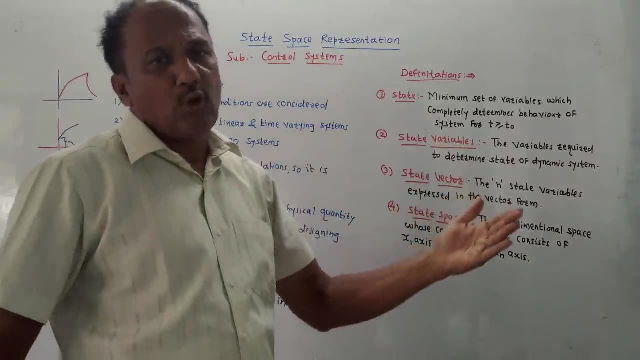 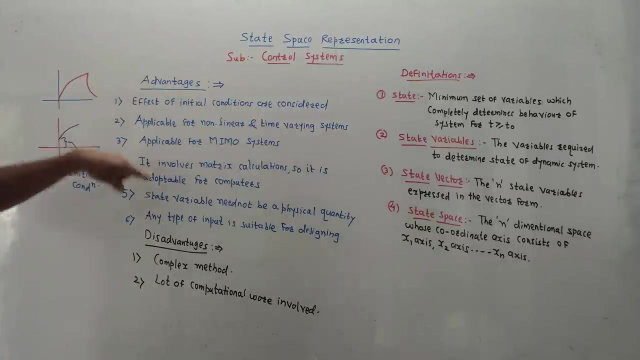 So advantages are effect of initial conditions are considered. Second: applicable for non-linear and time-varying systems. The conventional methods which we have learnt in other units. those are not applicable for non-linear and time-varying systems. This is applicable for such systems. Third, applicable for MIMO system. 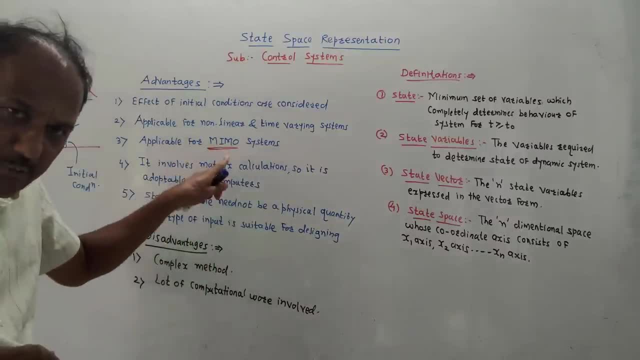 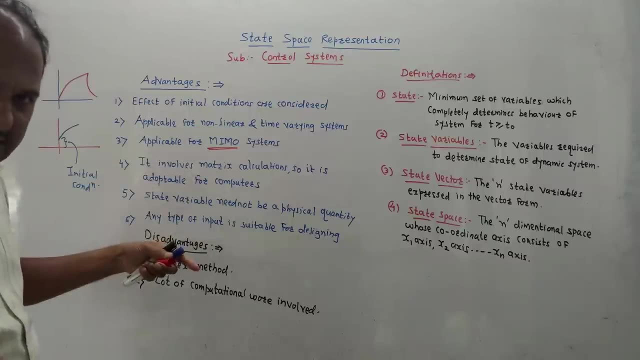 This MIMO stands for Multiple Input. Multiple Output system Means many inputs and many outputs. are applicable to any system, Then also this kind of analysis can be used. Next, it involves matrix calculation, So it is adaptable for computers. Next, state variable need not be a physical quantity. It can be anything. 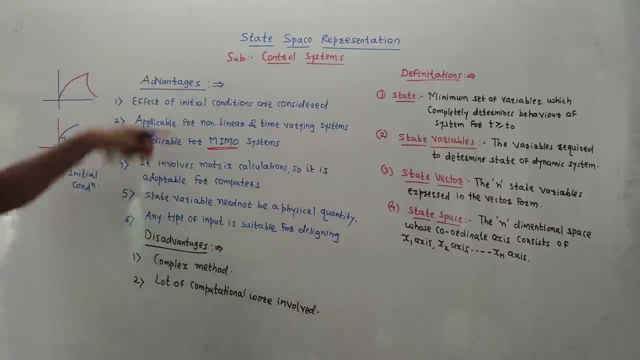 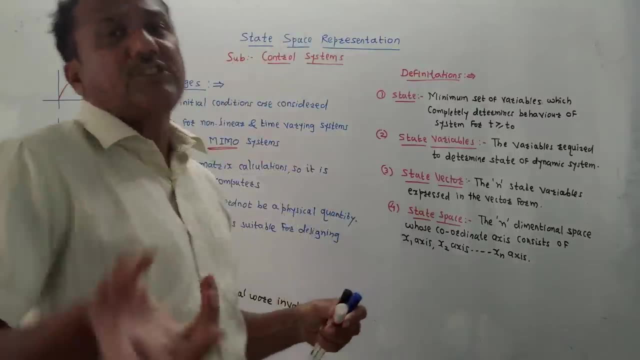 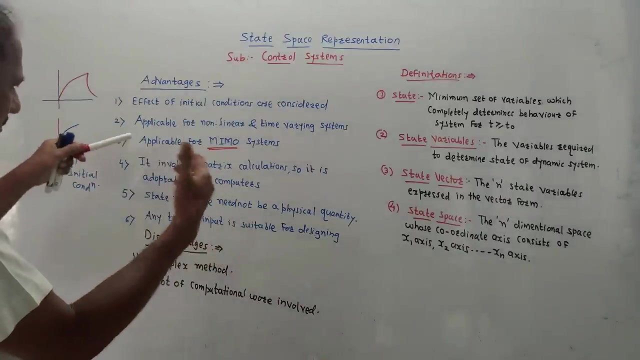 Any type of input is suitable for designing. So these are few advantages of state-space representation. If there is a question in the exam, what are the drawbacks of conventional control method? So these are the drawbacks of conventional method. For example, conventional control method cannot be used for non-linear and time-varying systems. 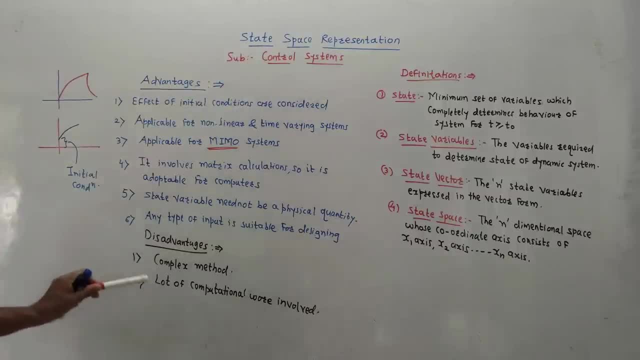 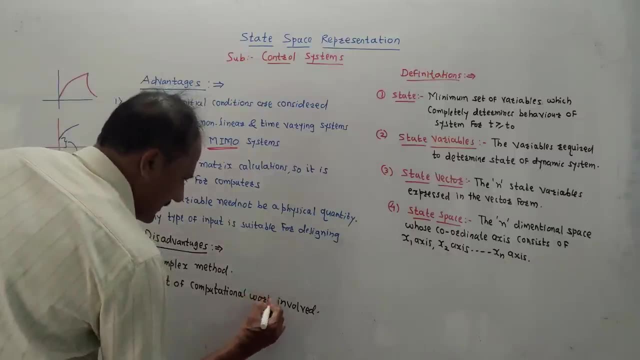 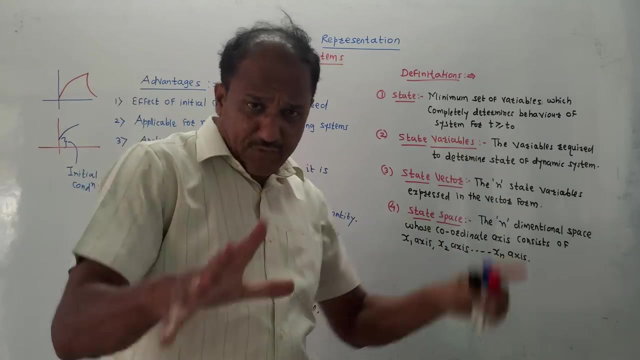 Now disadvantages of this state-space representation. First is it is a complex method And second is lot of computational work is involved. So if we solve numericals, these points will be more clear. Now we will discuss few definitions which are required for this state-space analysis. 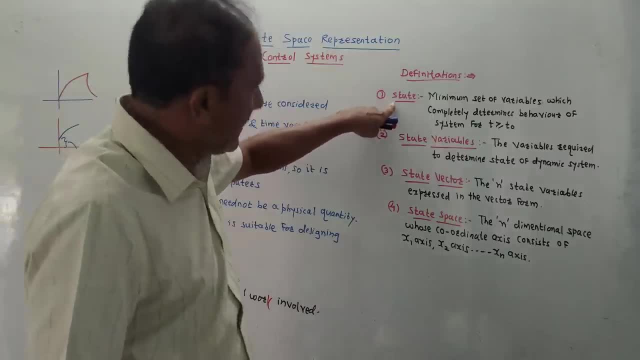 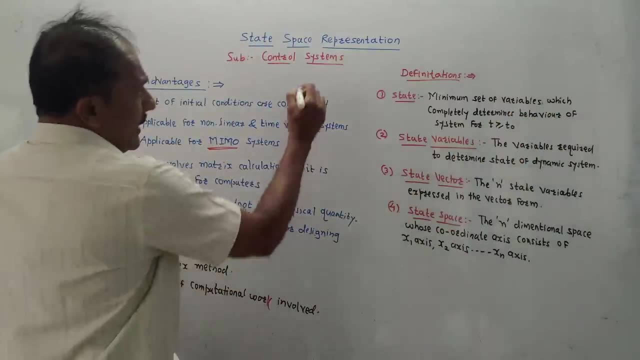 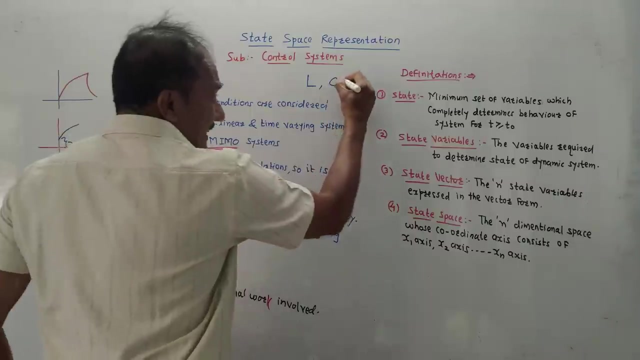 First is definition of word state Minimum set of variables. Now, what are these variables? Remember the basic concepts. We will be talking about two important components. One is L, that is, inductor. Second is capacitor, denoted by C. In case of capacitor, voltage across capacitor is important parameter. 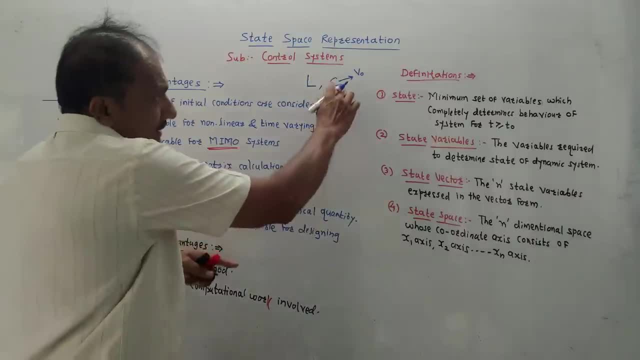 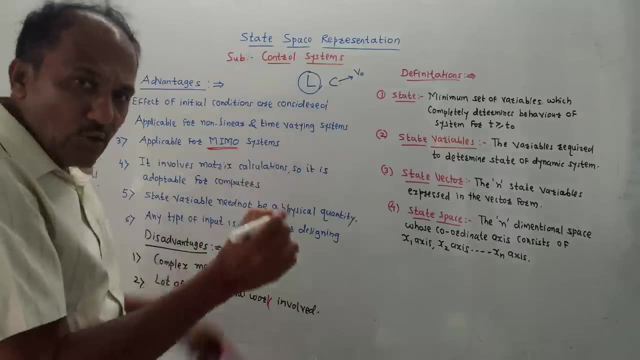 Capacitor is basically voltage control device. So if you are talking about capacitor, you need to take into consideration voltage, Whereas for inductor you need to take into consideration current, Because inductor is current operating device. So minimum set of variables: 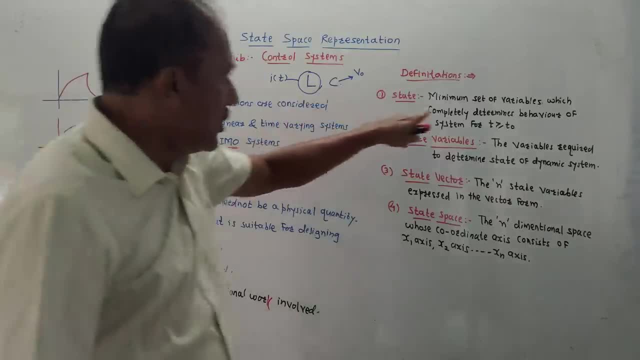 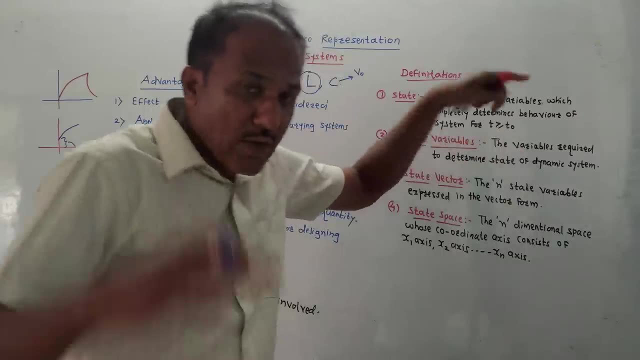 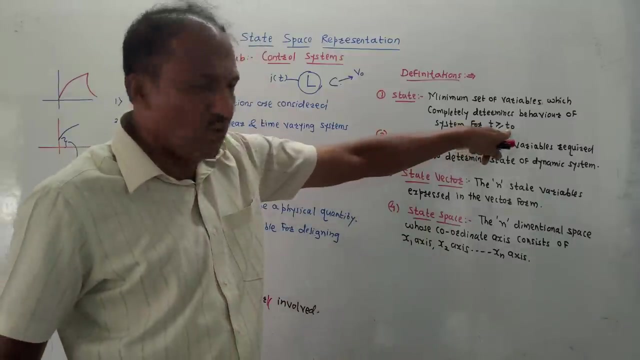 These are two variables. In circuit there is L and C, So minimum set of variables which completely determines behavior of a system For T greater than or equal to T0.. What is T0? The time at which we start an experiment. That time period is called T0. 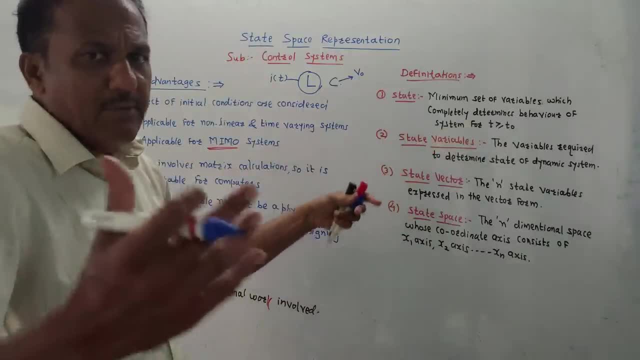 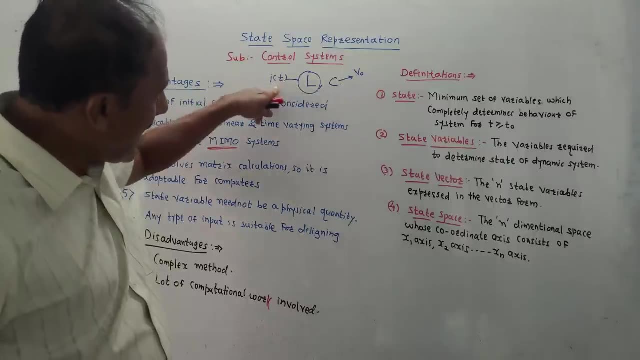 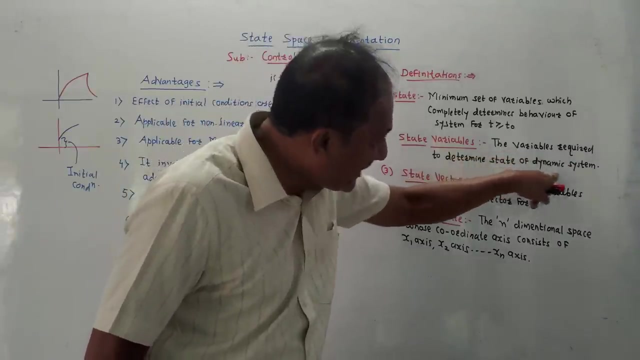 Now state variable. This is a variable Different notations are used to represent. For example, V0 is state variable which represents voltage across capacitor. I is another state variable Which represents current passing through the inductor. So the variables required to determine state of dynamic system is called state variable. 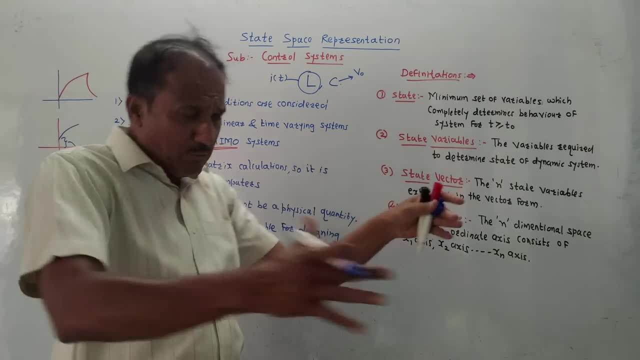 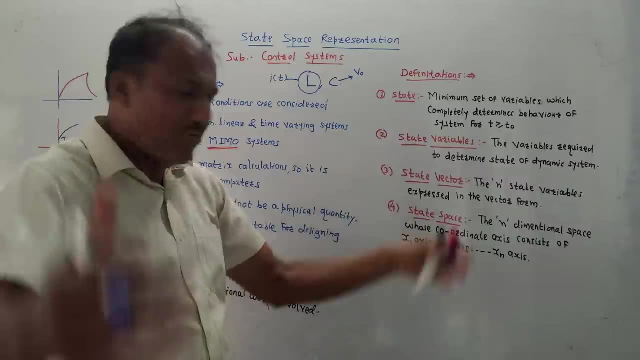 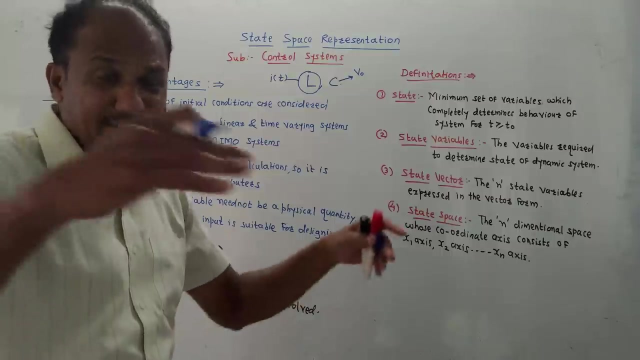 Next is state vector. It is very simple. We will discuss these variables more in numerical. These variables are expressed in the form of matrix, in the form of vector, So it is called state vector. Next is state space. Space means we will use different dimensions. 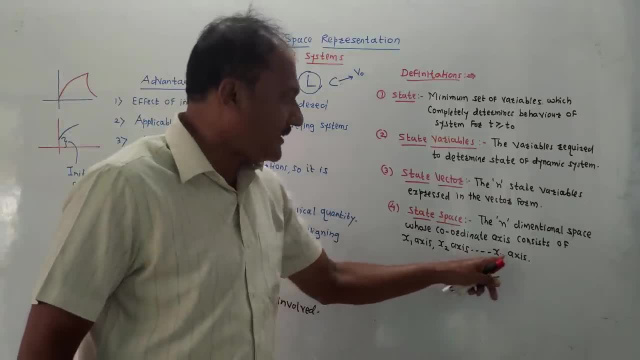 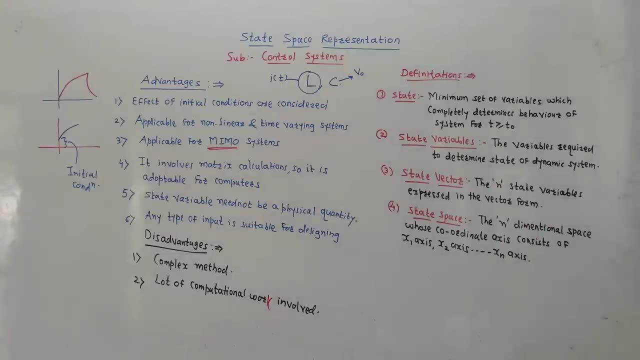 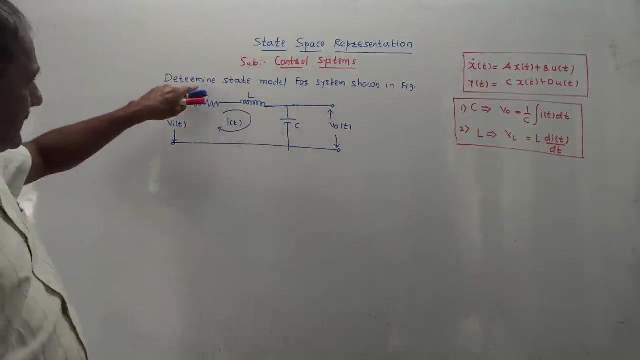 We will use different axes, Like X1 axis, X2 axis, Xn axis, So all these axes, Combination of all these axes is called state space. Now we will solve few numericals related to this state space analysis. First, numerical is determined state model for the system shown in figure. 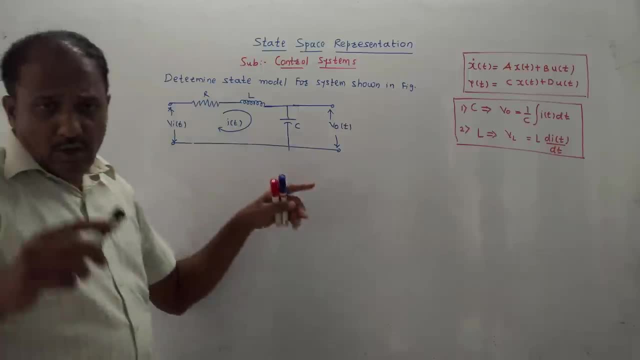 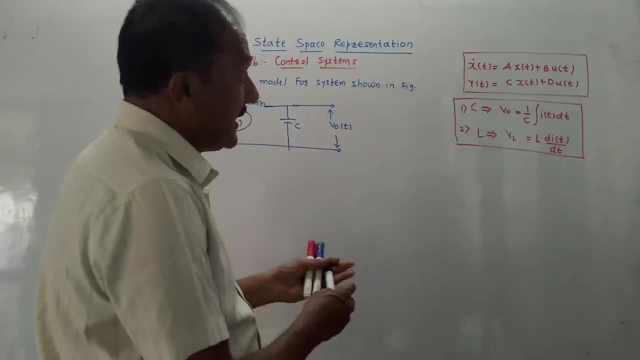 This is the given figure in the question. Now, see, We need some formulae, Basic formulae. Two formulas are required. First is X dot of T. Now question arises What this dot indicates. See, we have to remember very simple techniques. 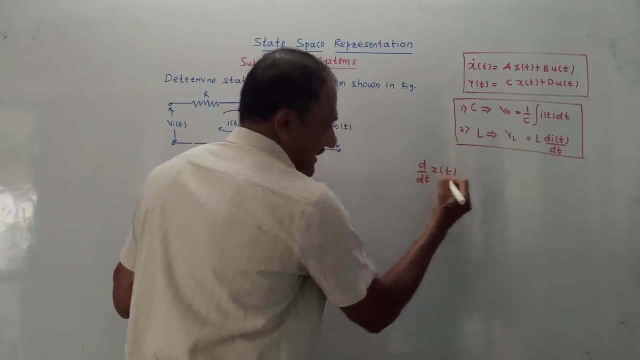 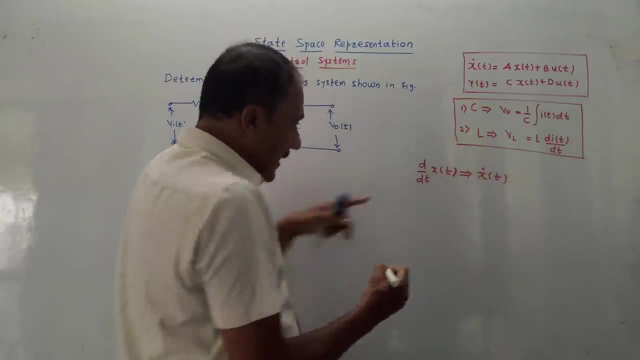 D by DT of X of T. This is how it is. In Maths we write like this: D by DT, Derivative of X of T. In this subject it is denoted by X dot of T Here if there is a double derivative. 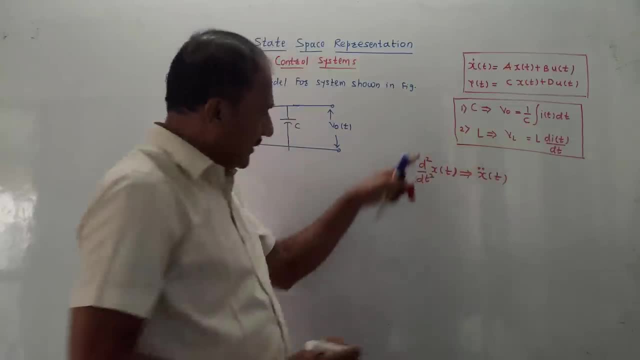 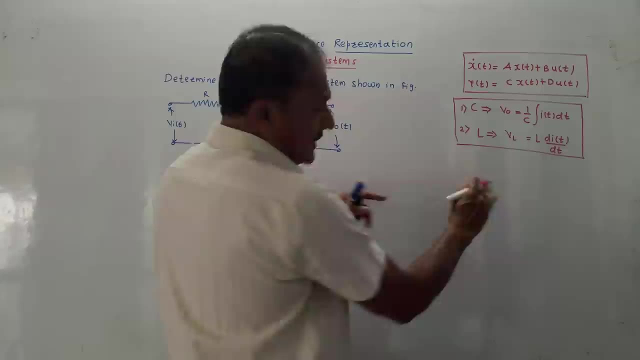 D square by DT square. So here we will write X dot. If it is D cube, then X triple dot, Like this. So this is the meaning of X dot of T. So formula is Means how to represent state model. There are two formulas. 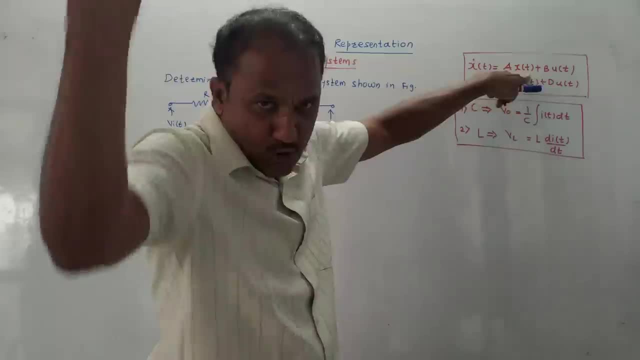 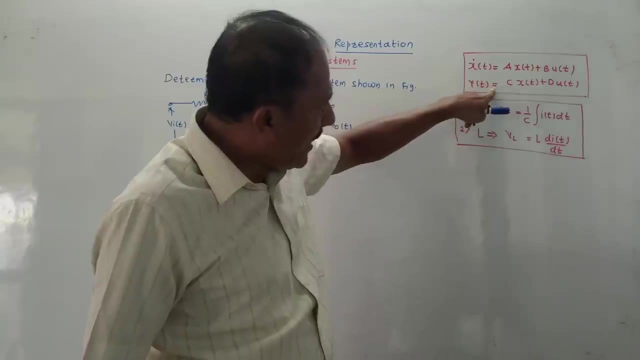 X dot of T is A, X of T. A means there will be some matrix that we want to develop, Plus B, B is again some another matrix, U of T And output Y of T is C, X of T plus D, U of T. 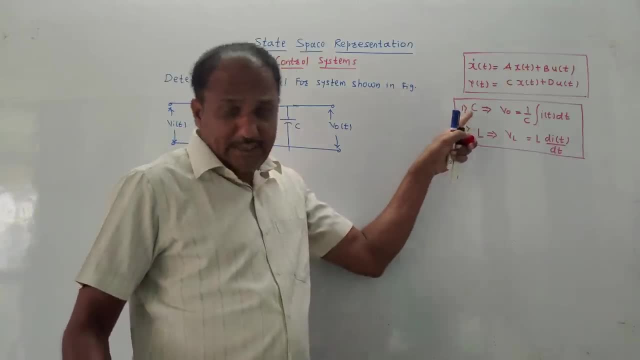 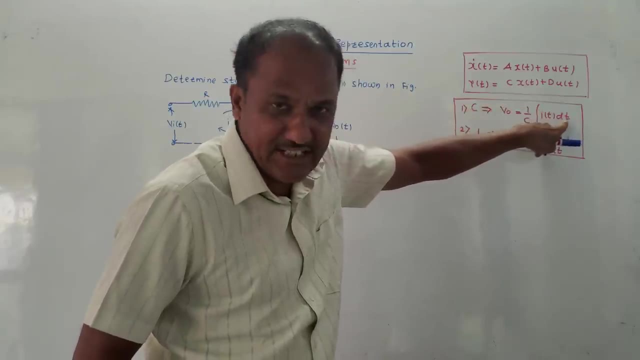 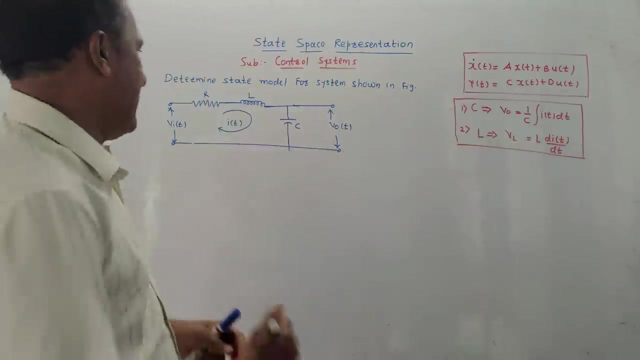 Now two more formulas are required. As I just told you, Capacitor is voltage operating device. So voltage across capacitor is 1 by C integration of IT DT. Then second for inductor, Voltage across inductor is L DI by DT. These two formulas are required. 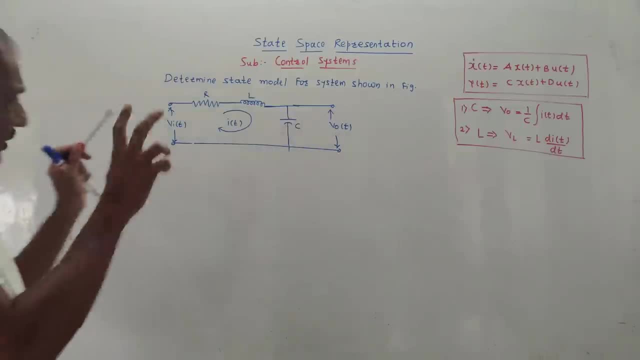 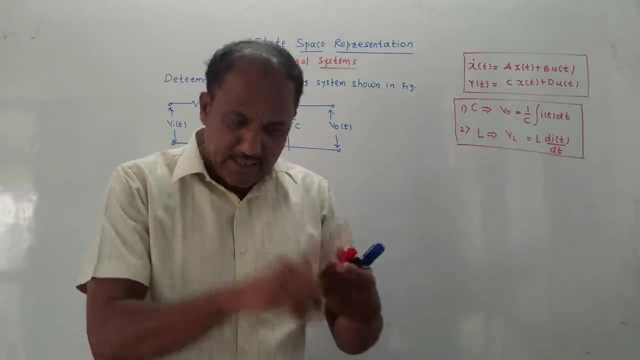 Okay, So this is the given question. Now you have to think like this: What are the storage elements in the given diagram? Look, Do remember the basic things. Register is not a storage element. Inductor and capacitor are storage elements. So L and C are storage elements. 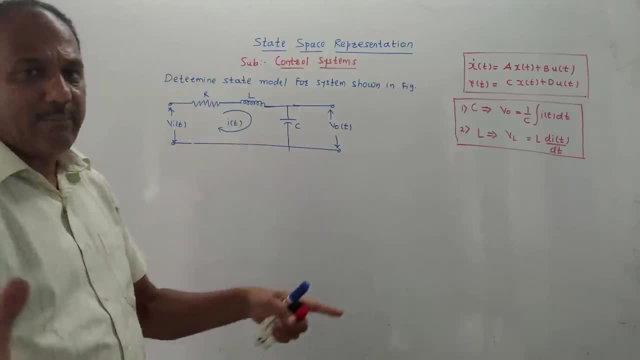 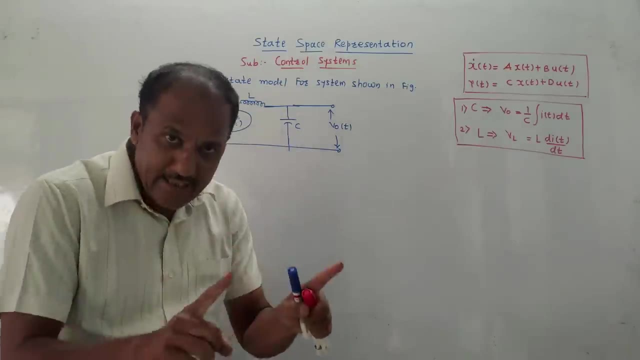 From the storage elements. state variable has to be assigned there. So I will be assigning state variable for L and C. As I just told you, Inductor L is current operating device. So in case of inductor I of T, Capacitor is voltage operating device. 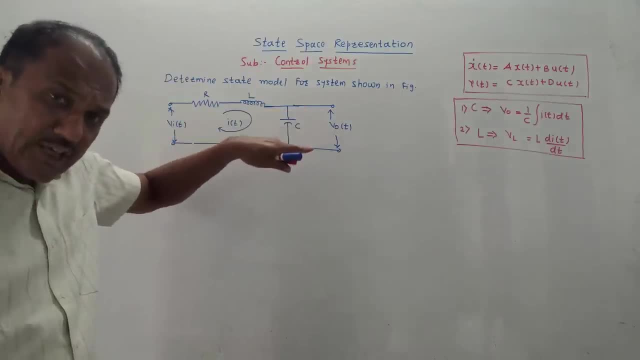 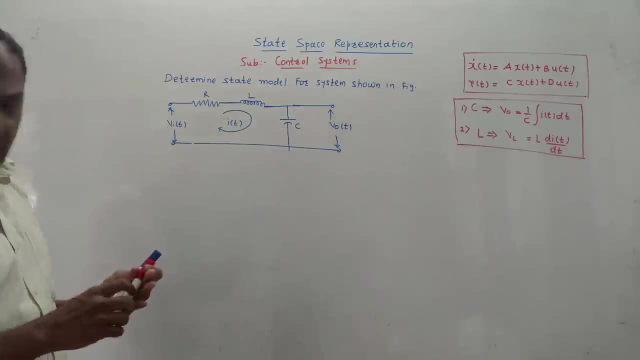 So in case of capacitor you should think of voltage In question. already it is mentioned. Voltage across capacitor is V, 0 of T, So state notation, Meaning how to assume state variable notation, By default input is given as VI of T, So input is denoted by U of T. 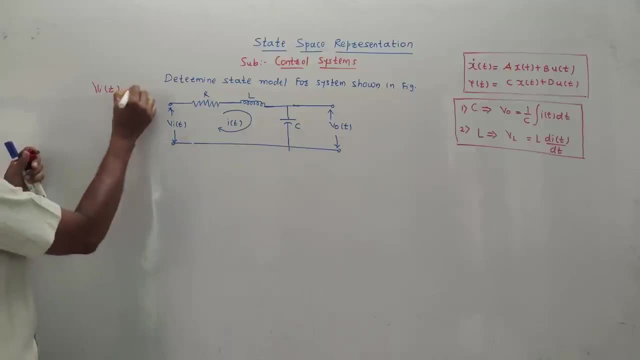 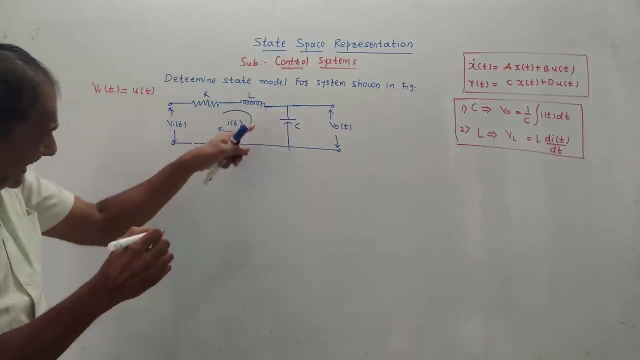 U of T is a state variable to be assigned for input. Second is the input, So the input is given as V? I of T. Second, Now, as I told you, Inductor and capacitor storage devices are fixed. For input, state variable will be U of T. 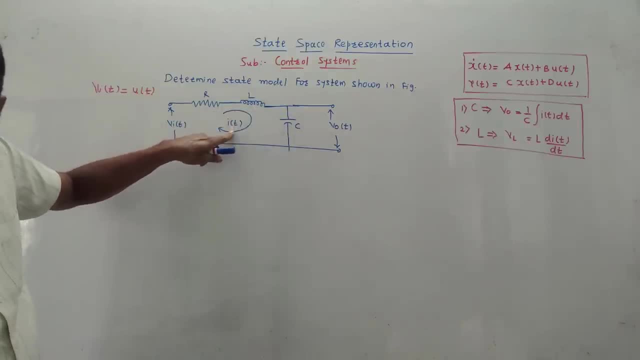 Rest the storage elements. For inductor I am thinking about current. So next state variable X1 of T is assigned for I of T. I of T is current through the inductor. As I told you, For inductor and capacitor state variable has to be assumed. 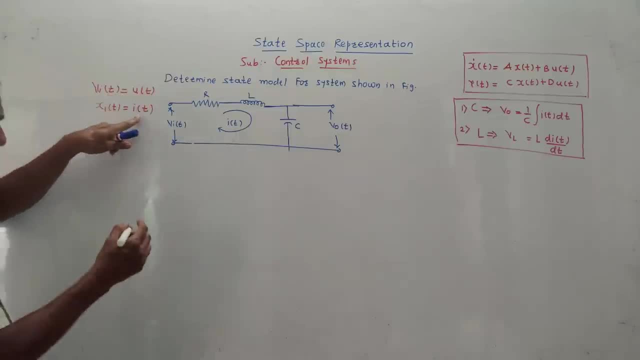 Rest, for input, fixed state variable is U of T. So for I of T I have assumed the state variable, notation X1 of T. Second notation X2 of T That we will be assuming for capacitor, Capacitor across, Meaning the voltage unit which is V, 0 of T. 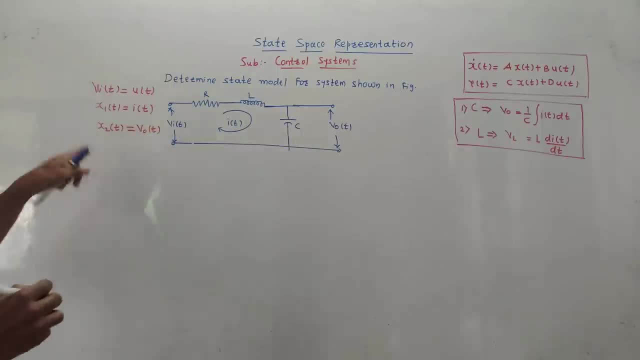 So that is represented by second state variable X2 of T. These are the notations. Now You need to apply a KVL See. Do not follow any lengthy techniques. Remember, KVL is simple. Input voltage is VI of T. 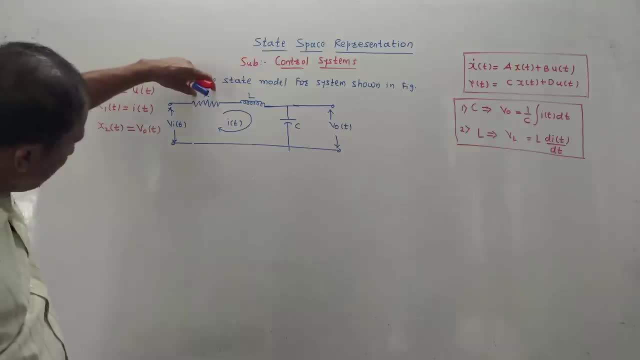 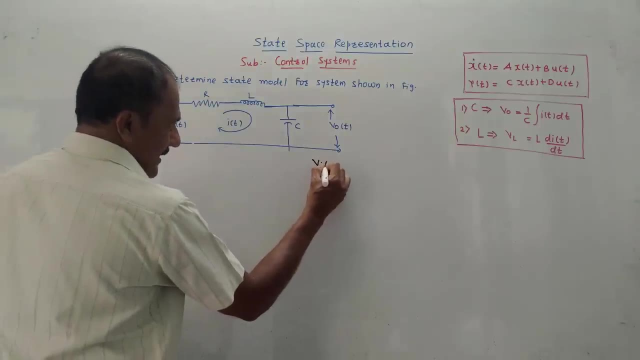 It will. It will create voltage drop across inductor, Across resistor, Across inductor and across capacitor. So in simplified language I can write like this: VI of T That is supplied, Applied input voltage Is equals to Voltage drop across resistor. 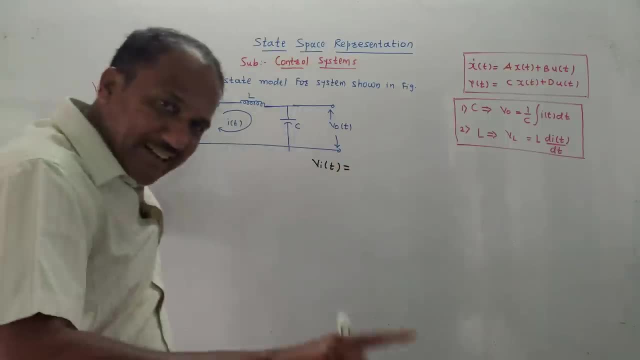 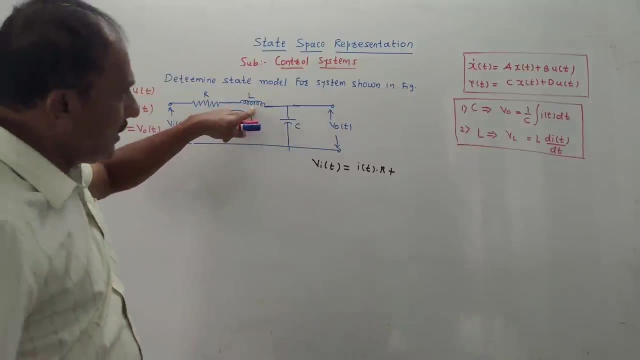 We know the formula Voltage drop across resistor is current into value of resistor, So I will write it as I: of T into R Plus Voltage drop across inductor. Its formula is L di by DT, So it is. 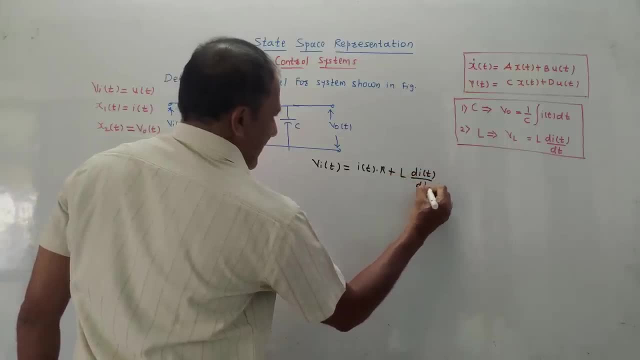 L di of T By DT Next Plus Voltage drop across capacitor. This is already given as V 0 of T, So I am keeping V 0 of T as it is. So this is simple. This is the application of KVL. 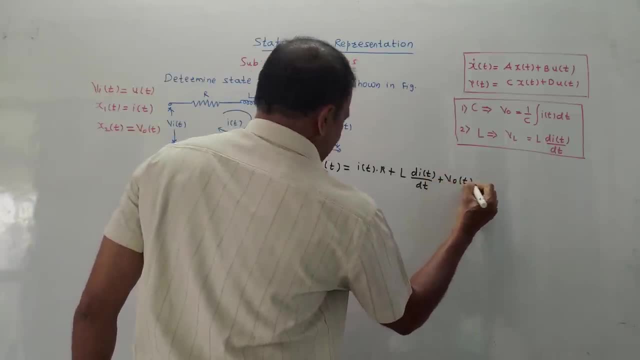 Input voltage, Whatever is available- Will be equals to Voltage drop across all elements in the circuit. So I have prepared an equation. Now You have to think like this: Where there is derivative sign That has to be taken in LHS. 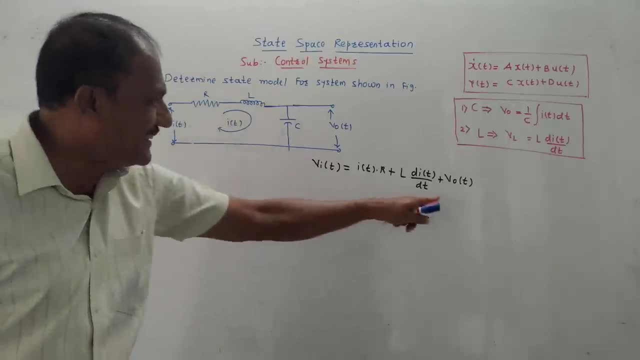 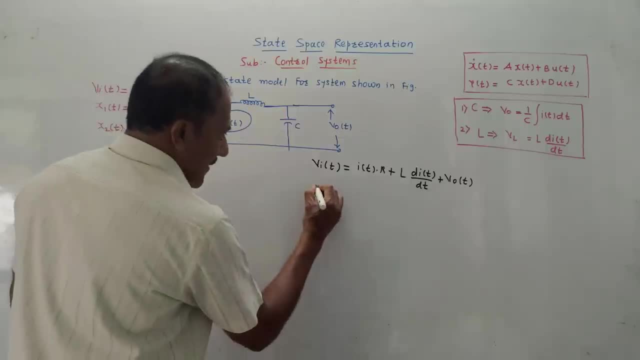 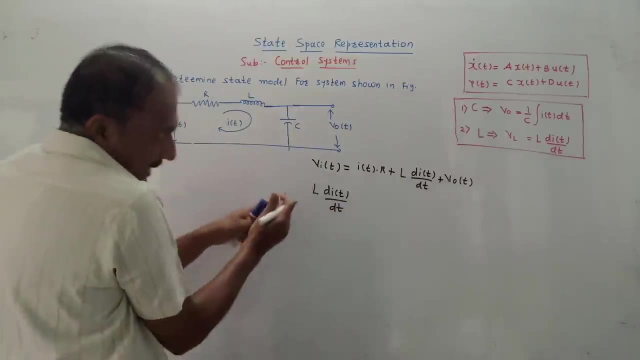 Now All remaining terms Have to transfer to RHS, So will rearrange the terms L, D, I, T By DT, Like I said, Where only derivative sign That has to be transferred to LHS, Remaining all terms. 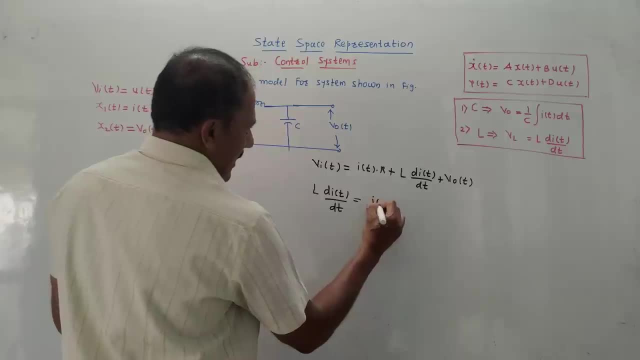 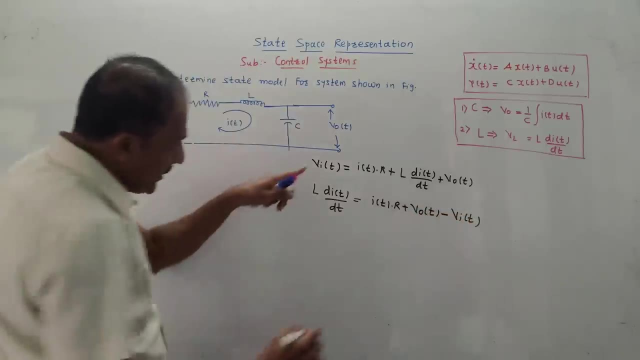 I will be transferring at the RHS. So it becomes I of T Into R Plus V, 0 of T Minus V I of T. Look Here: V? I of T Was in LHS. I transferred into RHS. 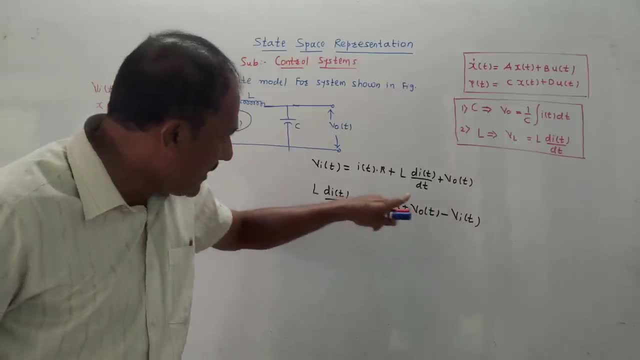 That's why it became minus And this term. This term Is equal to R plus V, 0 of T, Minus Vi of T. This is, If I am transferring at the LHS, it becomes minus. So this will be minus. 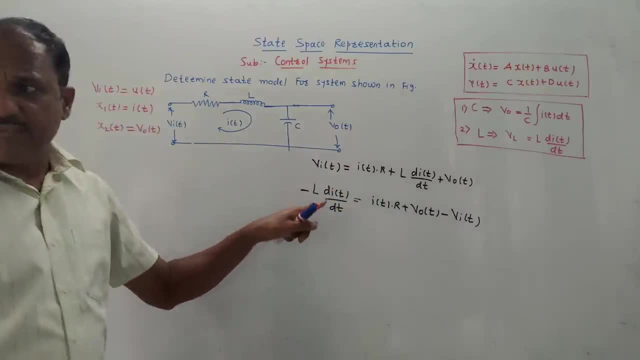 Rest the equation as it is. Now I have to assign the state variable. Now how to assign? See for I of t. what is the state variable? X1 of t? This is d by dt of I of t. 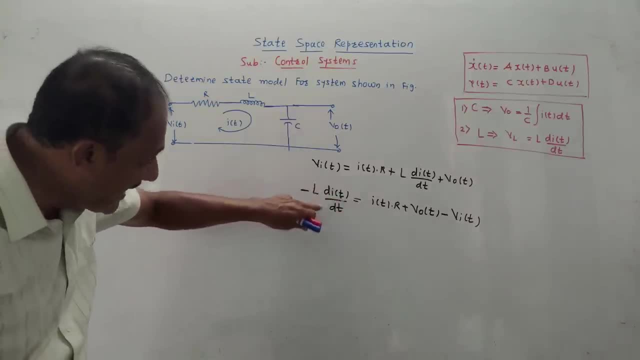 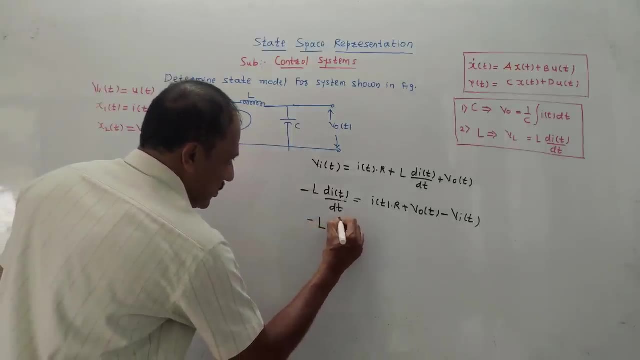 Means in return of I of t, I will be putting X1 of t, But d by dt of X1 of t is X1 dot of t. So this equation, I will write it as minus L: X1 dot of t. 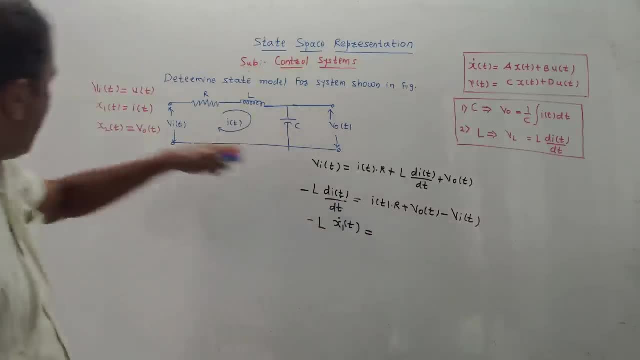 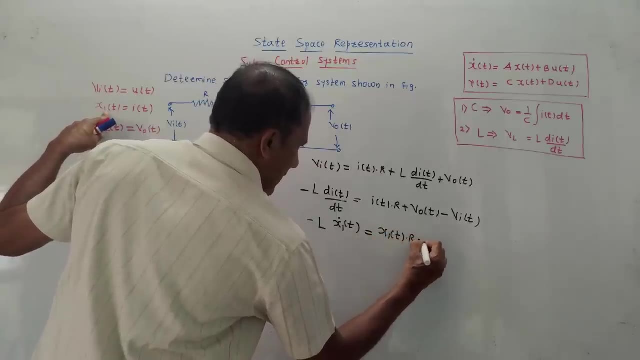 Equals to I of t. For I of t we have to see again. For I of t the notation is variable is X1 of t. So it is X1 of t into R Plus V0 of t. For V0 of t the variable is X2 of t. 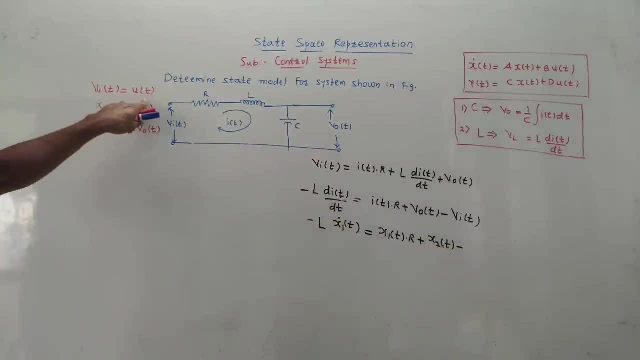 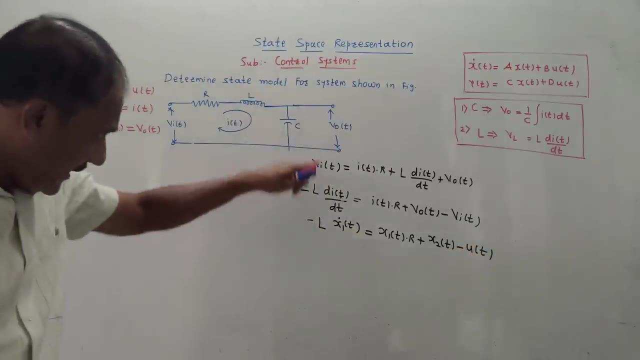 Plus X2 of t, Minus for Vi of t, the variable is U of t, U of t. So what I did? I have just written the values in terms of state variables. Now how do we think about the next step? 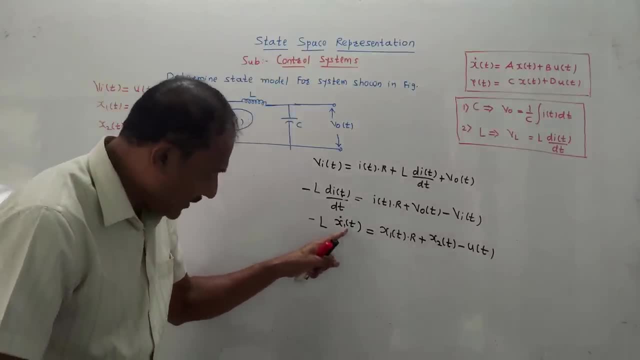 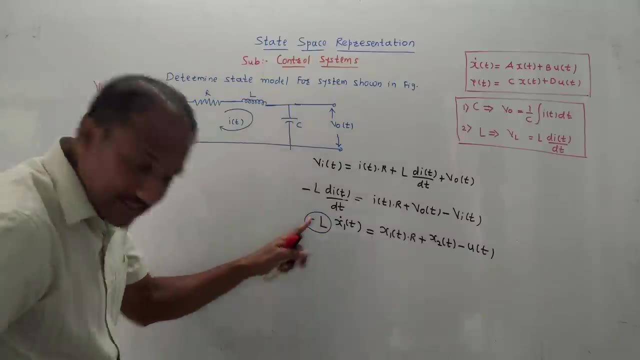 Only X1. dot of t means the derivative sign, Only this sign. Should we add the LHS? So I need to transfer this minus L to the RHS. I am transferring it along with minus sign. So next equation, I will write it like this: 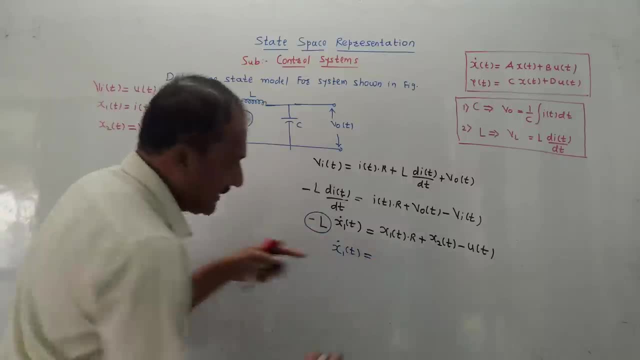 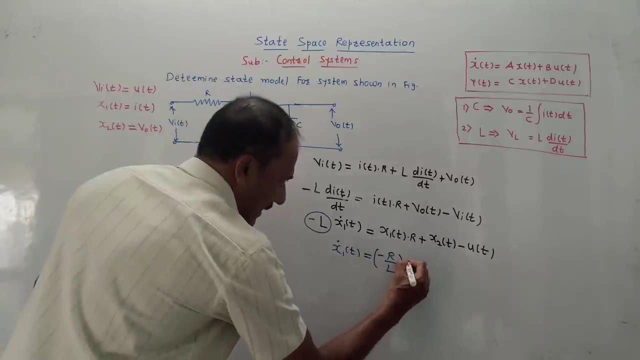 X1 dot of t is equals. to See, I am transferring minus L to RHS, So I will write it: minus R by L. Actually it is upon minus L. I have written it for simplicity. Minus R by L, X1 of t. 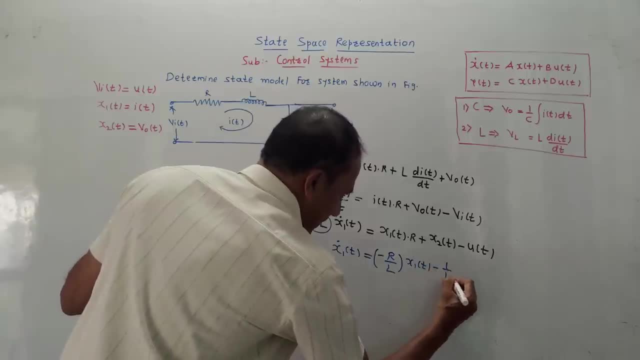 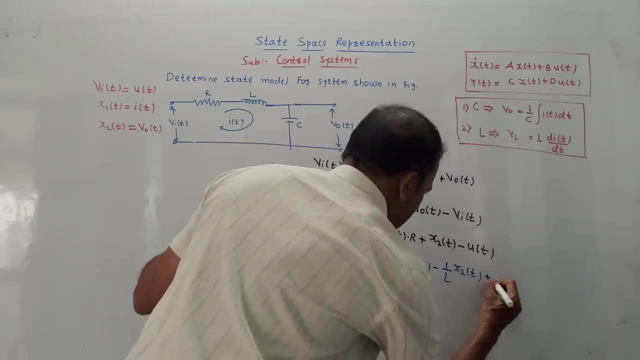 See this term When it comes to RHS. it becomes minus 1 by L? X2 of t. This is already minus sign and this is minus L, So it becomes plus 1 by L? U of t. So this is plus 1 by L? U of t. 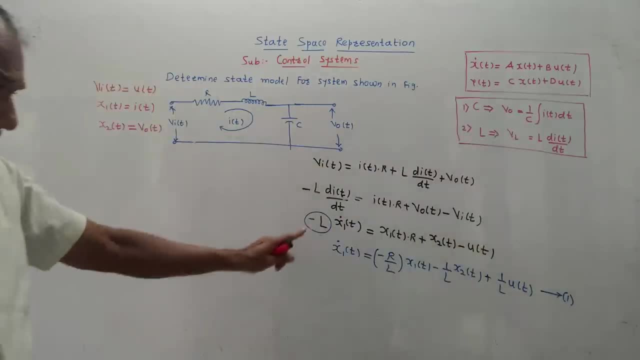 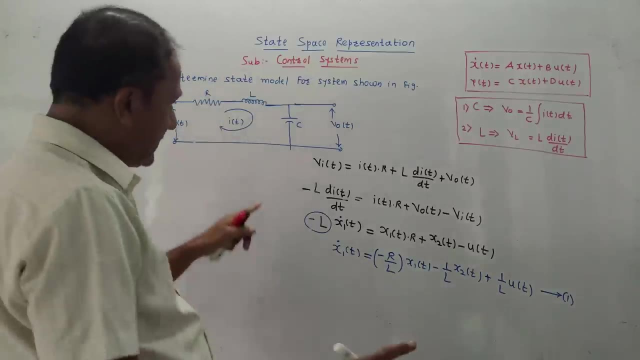 Let us say this is equation number 1.. How did I obtain equation 1? By considering input voltage. I have just applied KVL and and Avoid common mistake While preparing equation 1,: voltage across capacitor. this formula should not be used. 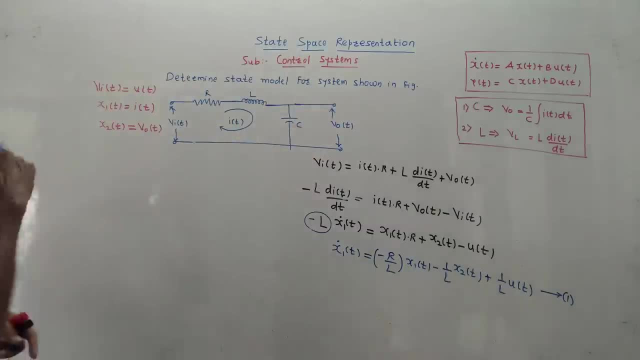 Use the generalized notation, that is V0 of t. Okay, This is equation number 1.. Likewise, I have to create one more equation. So see: output is denoted by Y of t. In this case, output is given as V0 of t. 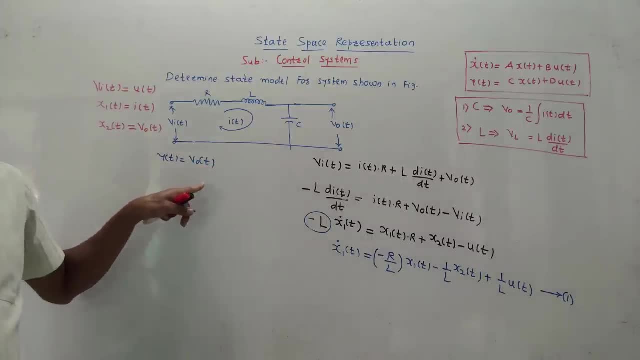 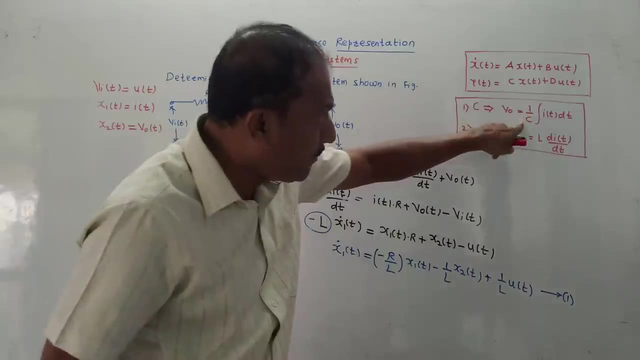 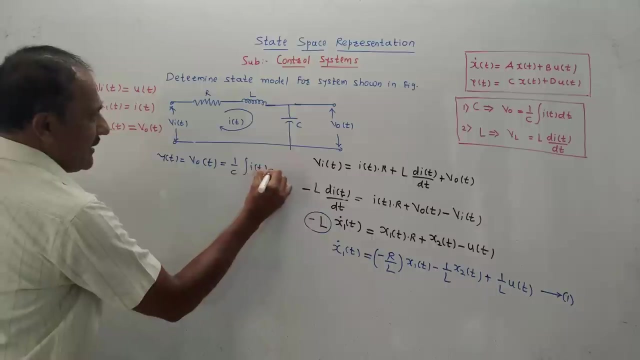 So output: general: notation is Y of t. In this case, notation is V0 of t. This is V0 of t And this is the voltage across capacitor. This formula is 1 by C, So it is 1 by C. integration I of t- dt. 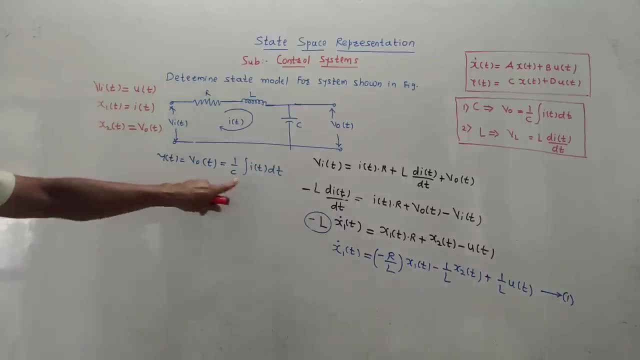 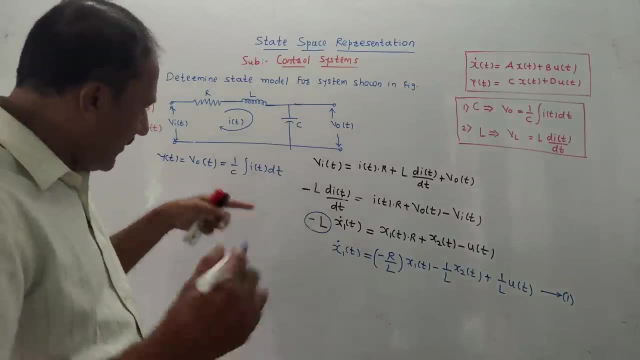 Now we have to think like this: I have prepared the general equation of this output. Now I want to cancel out this integration set. How to cancel the integration, Everyone knows: Take derivative of both sets. So if we will take derivative of both sets, 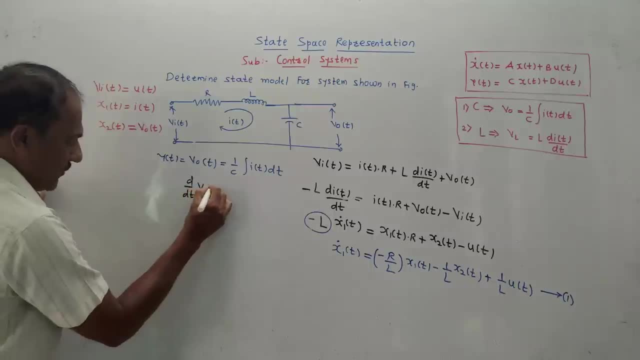 it becomes: d by dt of V0 of t is equals to 1 by C, Integration and derivative set is left I of t, Now d by dt of V0 of t. Think about this: V0 of t means: 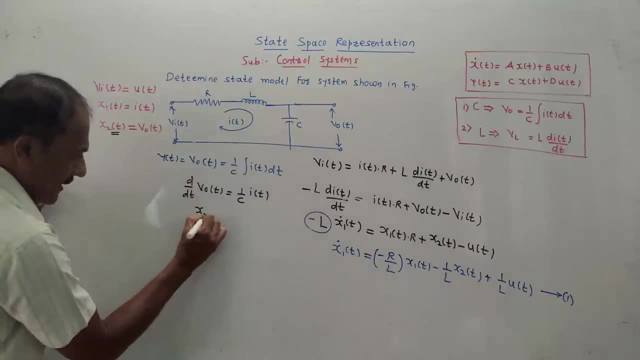 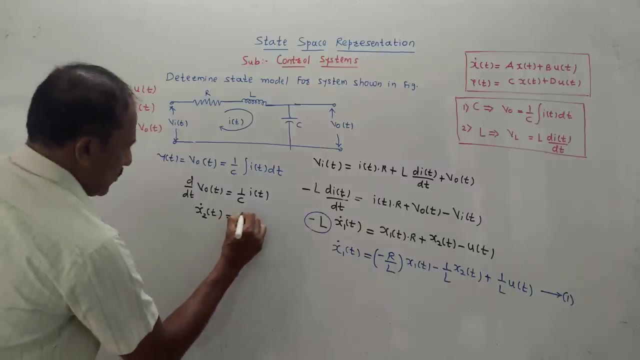 X2 of t and d by dt of X2 of t it becomes X2 dot of t. So for LHS I have written: X2 dot of t is equal to 1 by C I of t. What variable have we used for I of t? 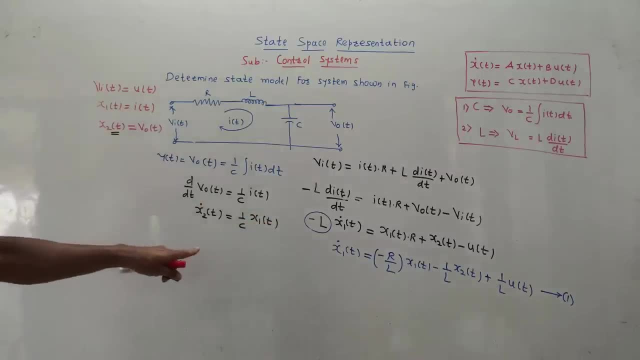 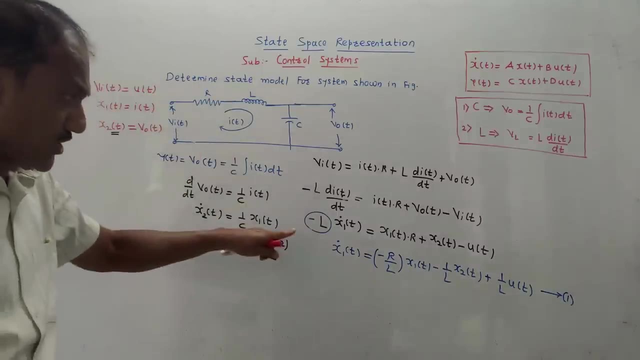 X1 of t, X1 of t. This is equation number 2.. So see state variable says so. I have created two equations, equation to cassette. I can simple by considering the equation of output- equation- one cassette there here- by considering input applied to the system and by applying KVL. so we have 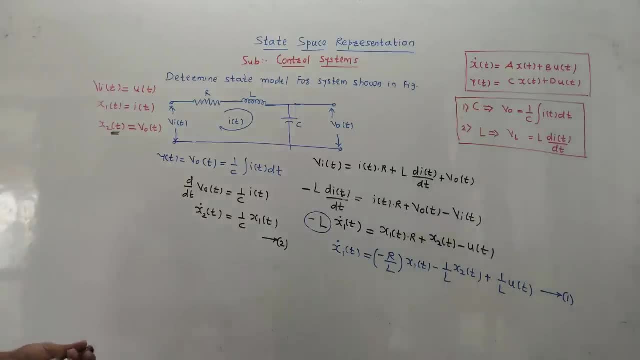 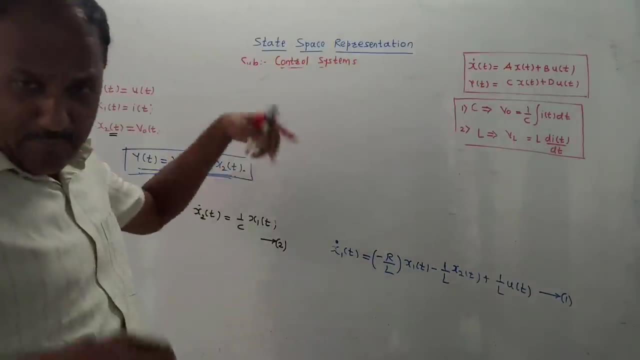 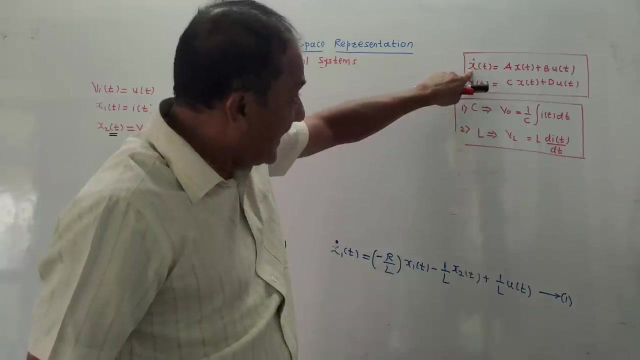 these two equations. now, by making use of these two equations, I will have to create the matrix. now, last step of this numerical, I will have to create the state model. but the matrix are connected by making use of these two equations. at the LHS I have X, 1, X, X dot of T, but we have two variables related to X, dot of T. 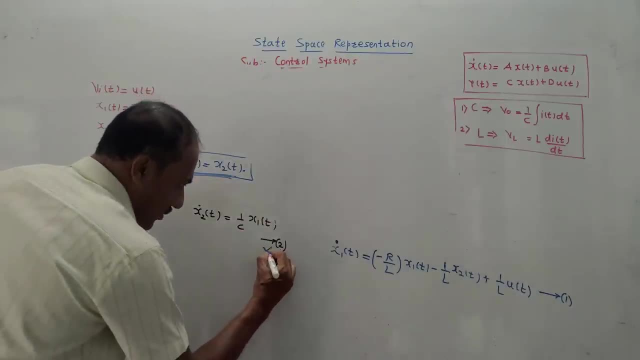 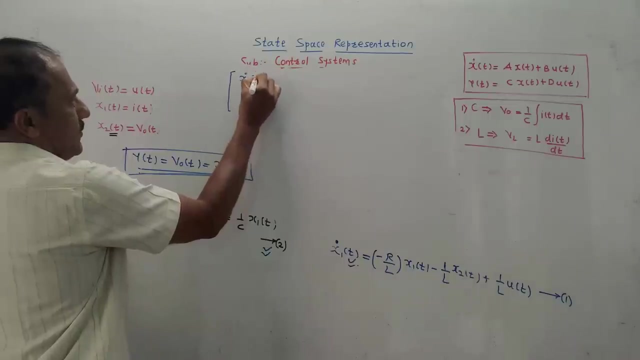 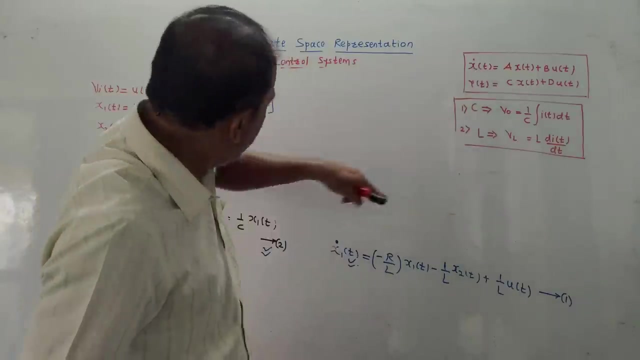 that is X 1 dot of T and X 2 dot of T. so I will be making use of equations one and two. so LHS term it will be column matrix where I will be writing X 1 dot of T, X 2 dot of T. in LHS there is X dot of T. in this numerical there are two variables. 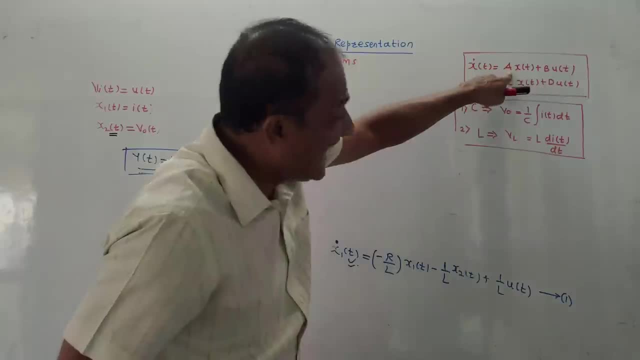 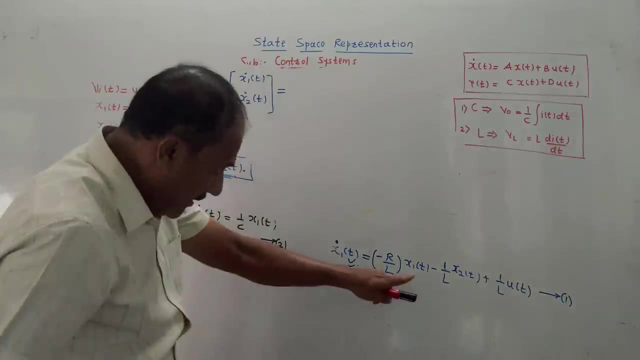 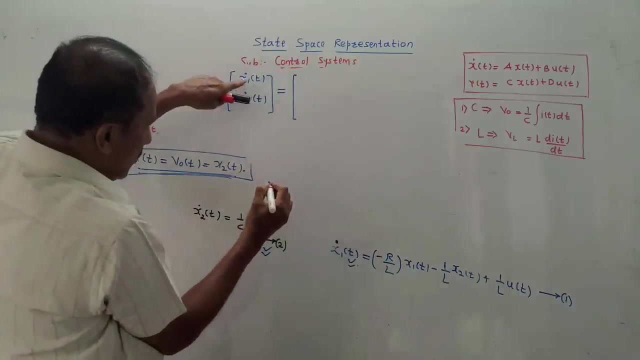 X 1 dot of T and X 2 dot of T equals to now we have to create matrix A. yet cassette air current A into X of TA. referee equations one and two equation one way: X 1 of T coefficient is minus R by L. so here the X 1 dot of T comma, the 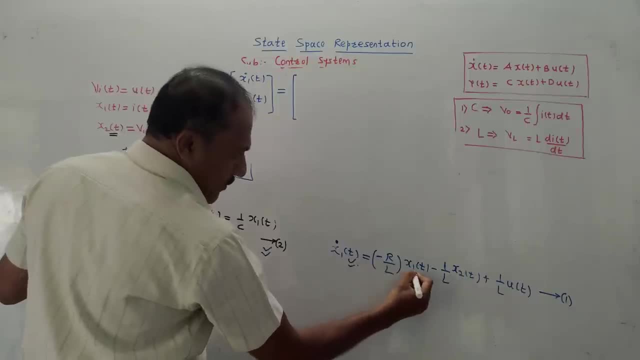 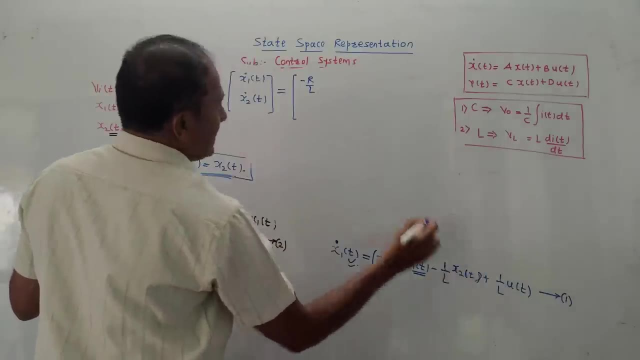 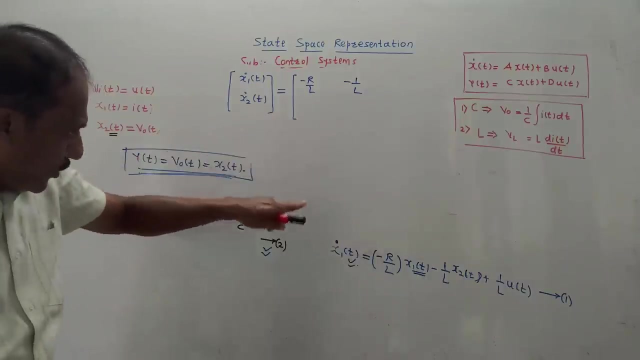 first row as a such night for X 1 dot of T. first coefficient for X 1 of T is minus R by N. for X 2 of T, this extra of T coefficient is minus 1 by N. to your bad Second row again, we will be referring to equations 1 and 2.. 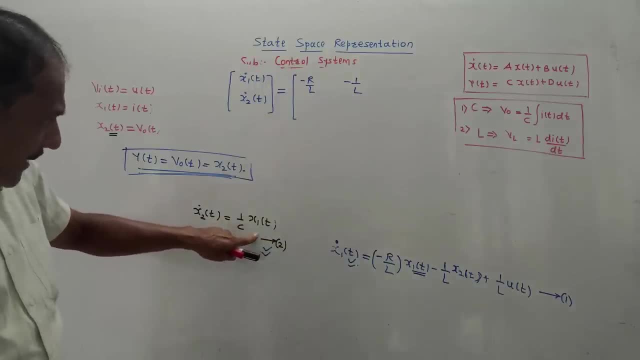 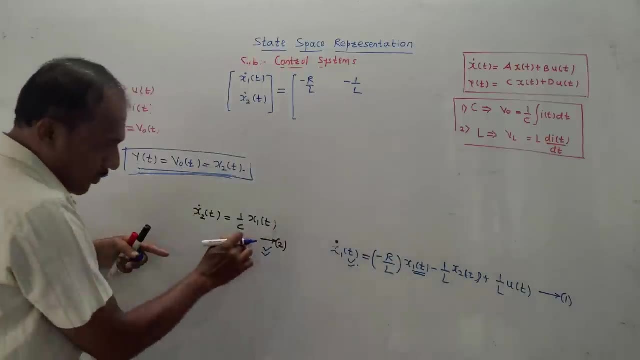 So in equation 2, the coefficient of x1, see. for second row, I have to refer to equation 2.. For the first row I have referred to equation 1.. For in equation 2, the coefficient of x1 of t is 1 by c. so here I will write 1 by c. 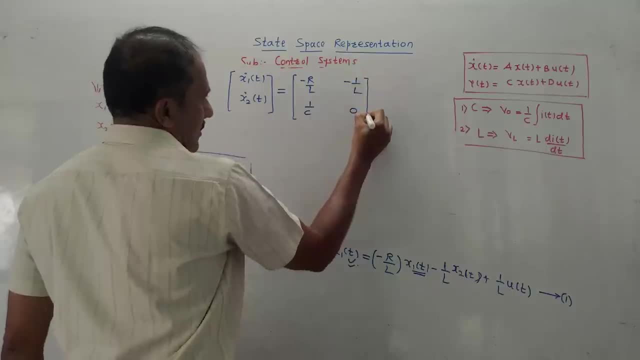 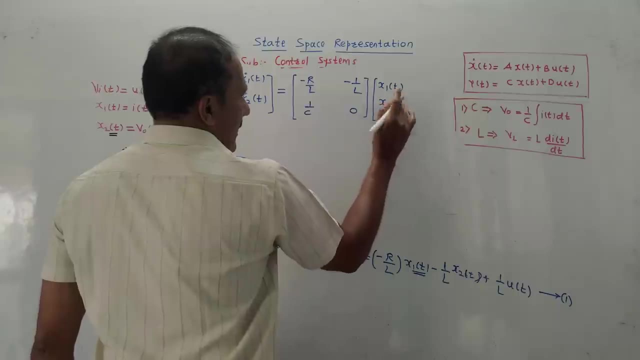 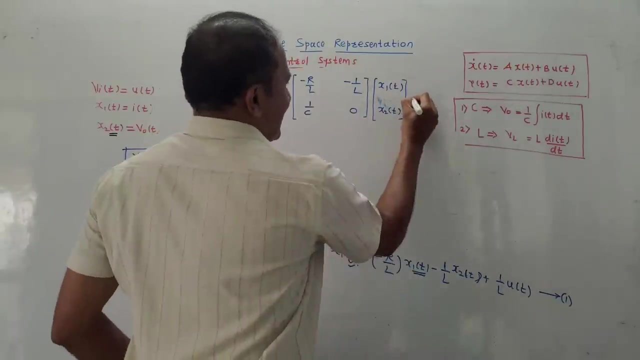 There is no x2 of t term, so 0. See a into x of t. So x of t means in this case it will be x1 of t and here I will write x2 of t. This is a into x of t. plus see the equation b into u of t means I have to make the b. 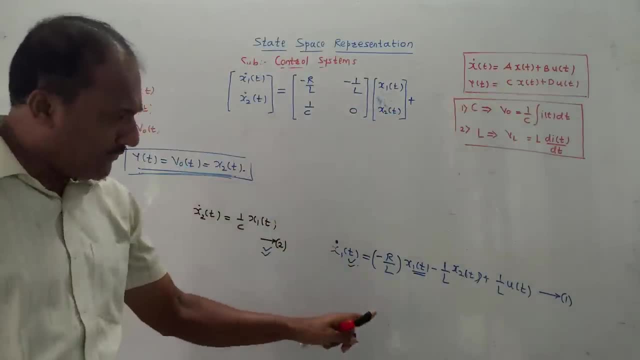 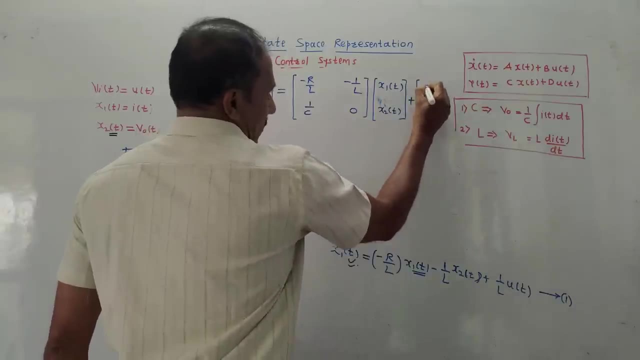 matrix into u of t. Now I have to refer to equations 1 and 2.. In equation 1, I have terms related to u of t whose coefficient is 1 by L. So I will be writing it like this: 1 by L. 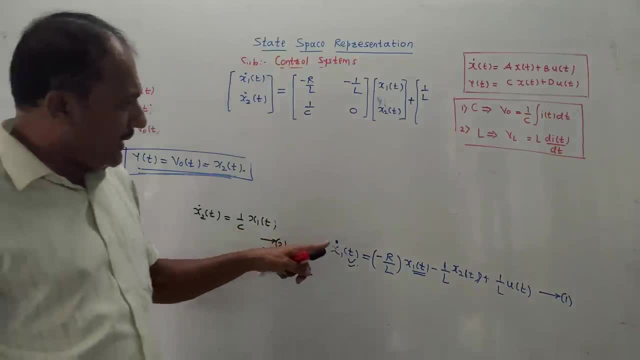 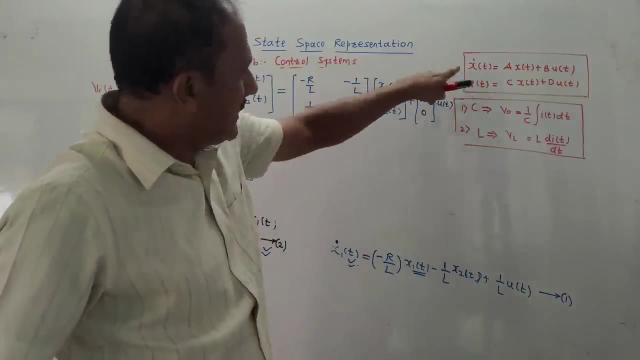 In equation 2, there is no coefficient related to u of t, So I will be writing it like this: 1 by L related to u of t, So it will be 0 into u of t. So this is the equation, this is the. 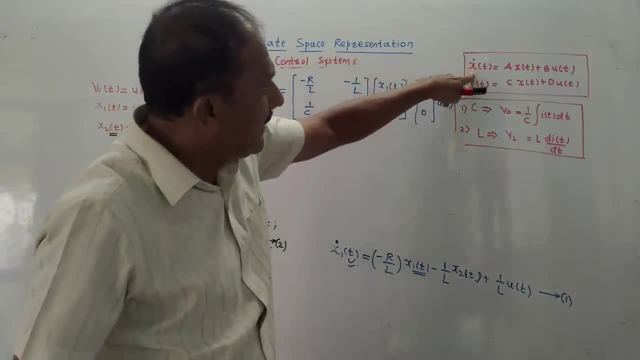 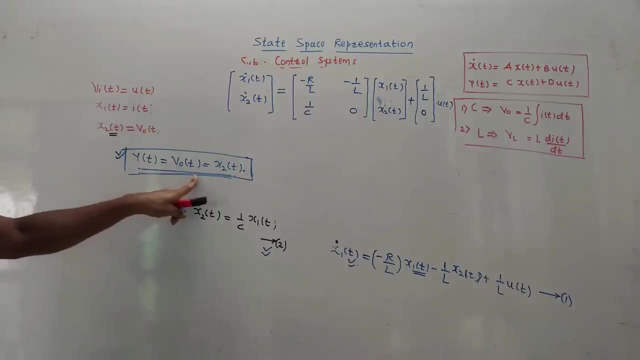 matrix representation, rather state model representation, related to x dot of t. Now we have to keep the output equation. This is the equation of output. We have already developed this equation. So how to make the matrix Refer this equation? So it is y of? 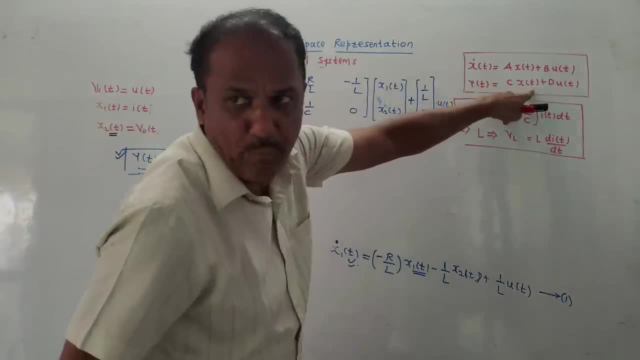 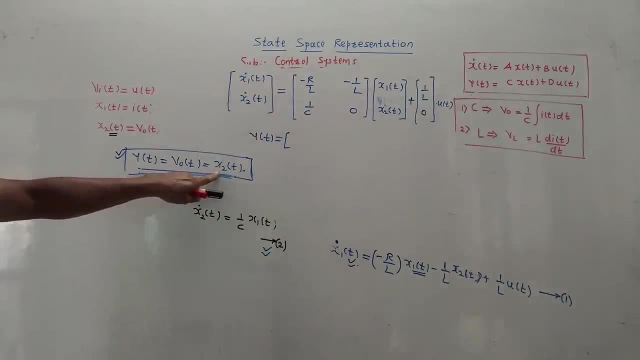 t is equal to c into x of t. So this matrix- this will be a row matrix. How to make this? I am referring this equation of output only In y of t. these two equations, one or two equations, are not to be referred. So y of t is x dot of t. So I will write 0, 1.. First, 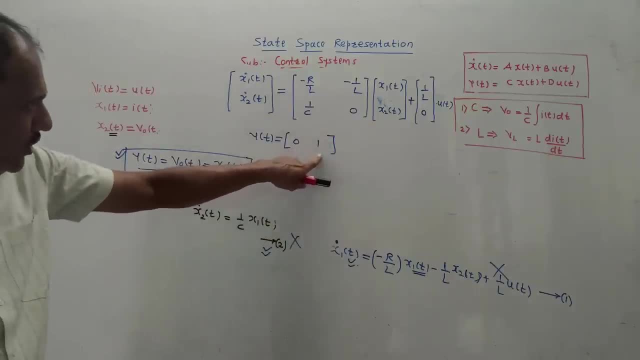 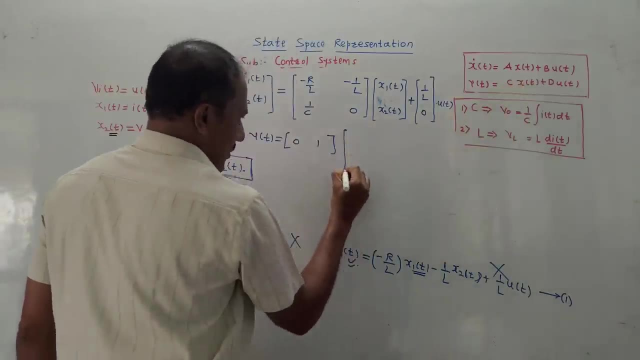 element. this will be for x1.. It is 0.. So I have written 0 for x. dot of t. Its coefficient is 1.. So I have written 1.. Thank you. format: they go c into x of t. x of t in this case is x1 of t and second term is x2 of t plus. 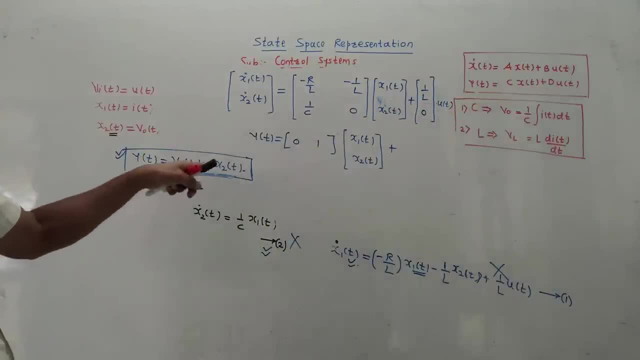 b into u of t. there is no u of t term in the equation of output, so simply i will write 0 into u of t. this is optional, you may skip it. so i mean about this last term. so this is called the state model representation of the given. let us solve one more numerical. next numerical is: 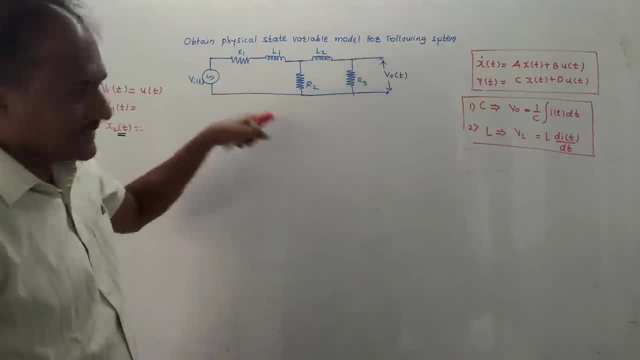 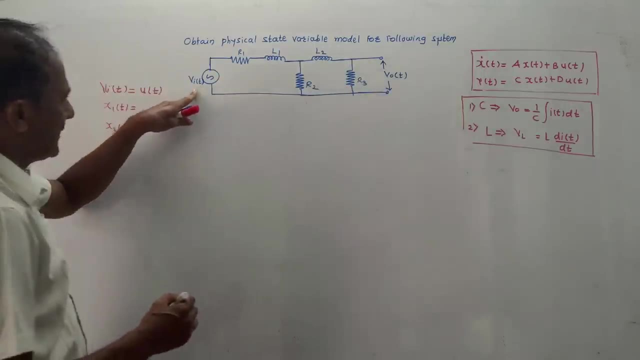 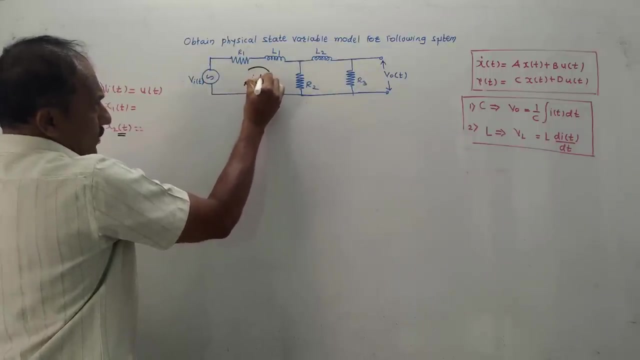 obtain physical state variable model for the following system. this is the given diagram. there are two loops actually. v0 of t is output voltage, v? i of t is input voltage. if the currents are not given in the question, like this: for first loop current is i1 of t. for second loop current is i2 of t. 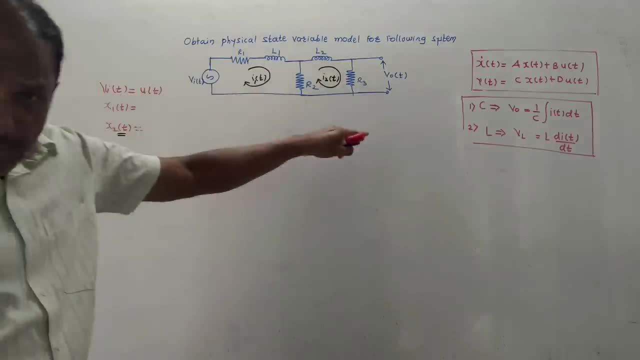 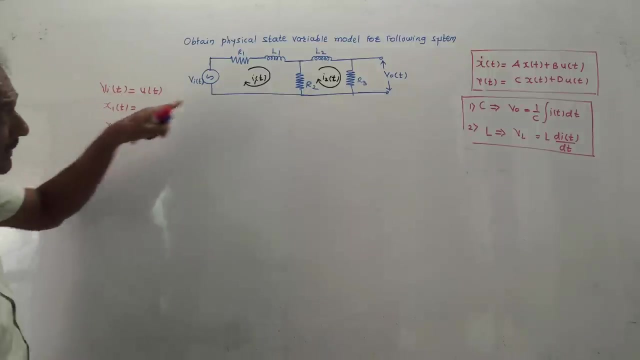 now there is no capacitor, only inductor. we know that inductor is a storage element. now how to assume the notation of the state variable. like the previous sum input v, i of t is assumed to be u of t means its notation is u of t. x1 of t means the first variable- see this- is inductor. in case 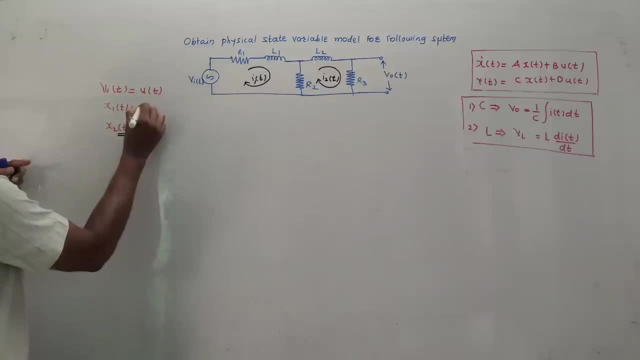 of inductor, we have to think of current. so first notation is i1 of t. that means x1 of t in place of i1 of t. i will be using notation x1 of t for x2 of t. notation will be i2 of t, living in place of. 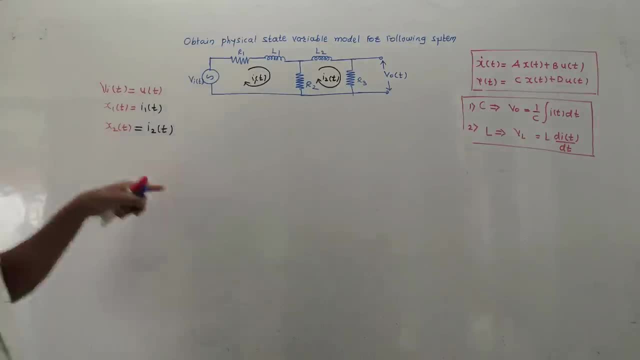 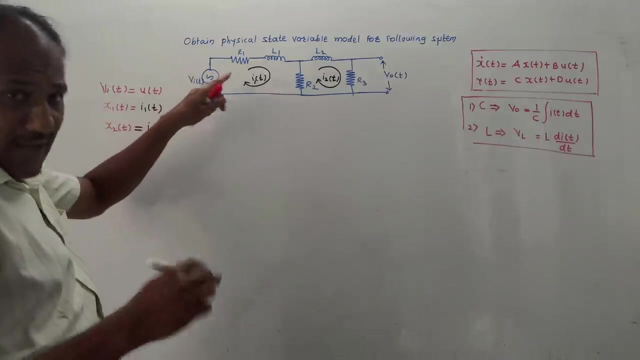 i2 of t. i will be using state variable like this. so this is the way how to write the equations. like the previous sum i will have to make. i will have to for first equations by using kvl. now for first loop, i'm telling you the. 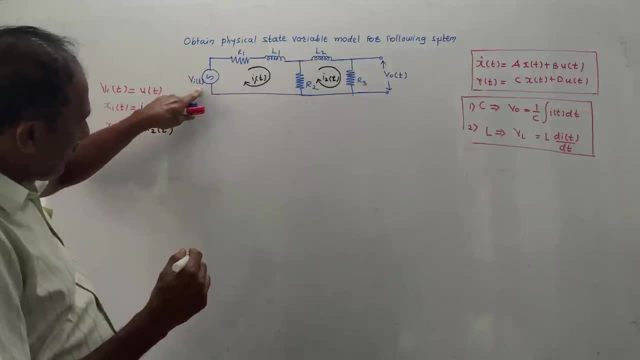 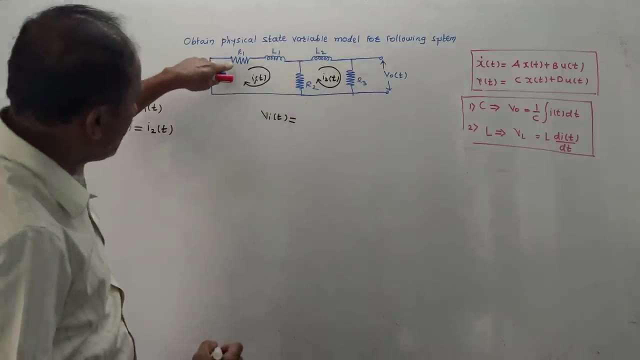 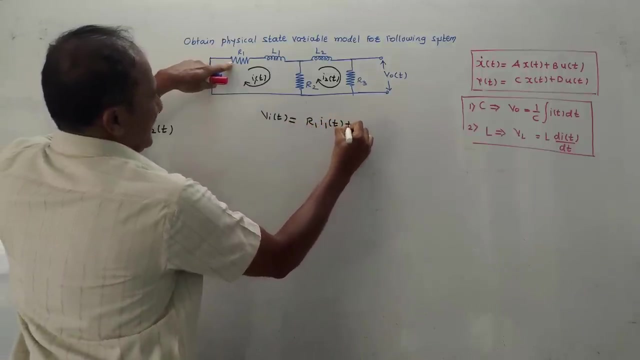 simplest trick. input applied voltage is v i of t. so first i will write: di of t is equal to voltage drop across all elements. So start from this is equal to R1 into I1 of t Plus. this is the inductor voltage drop across inductor. 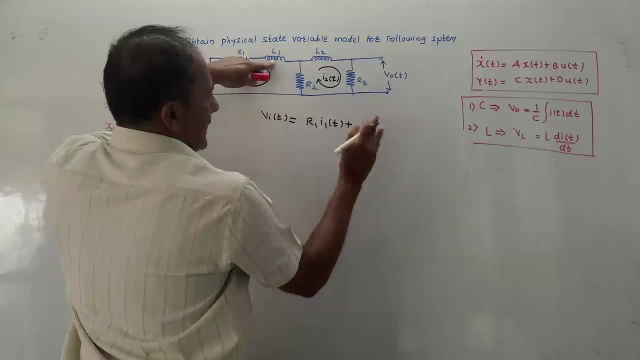 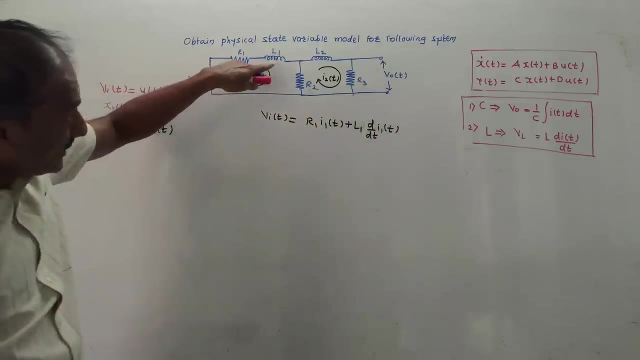 is L, di by dt, So it is L that is value of inductance, that is L1, d by dt of I1 of t. Do remember, through this L1, only I1 of t is flowing. Then come across this: 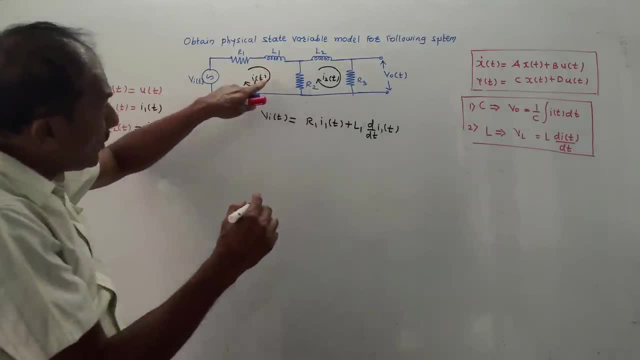 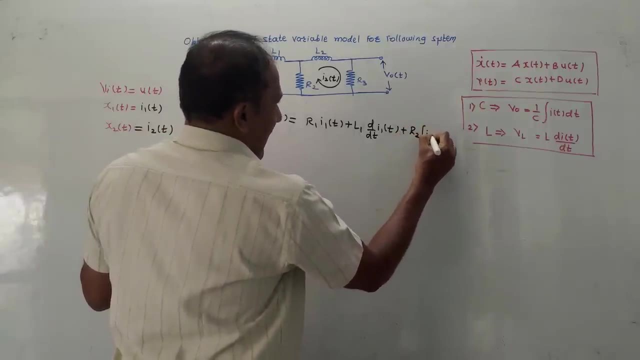 It is voltage drop across R2.. For R2, both currents I1 and I2, are flowing, So I'll be writing it like this: R2 in the bracket I1 of t minus I2 of t. You don't have to make a mistake here. 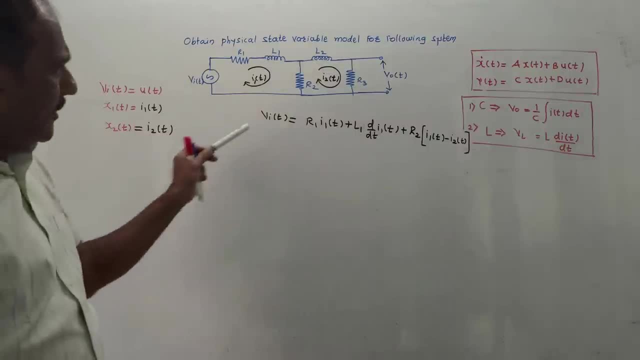 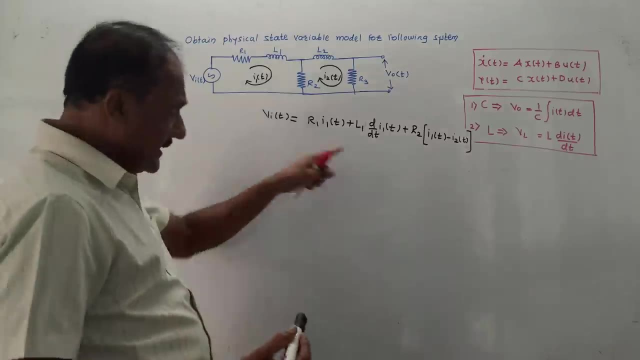 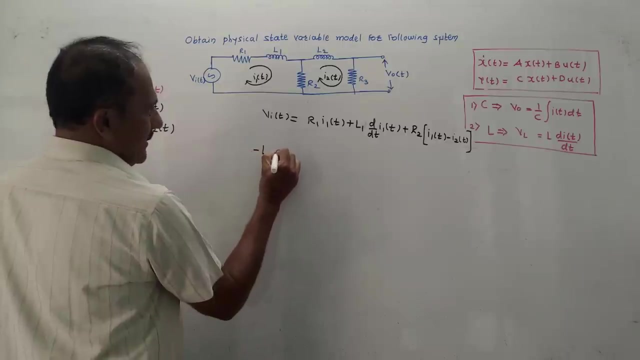 So this is the KVL, by considering only input loop. Now, like the previous term, I will have to rearrange the equation. How to rearrange the equation D by dt term? I want it in LHS, So I will write it like this: minus L1 d by dt of I1 of t. 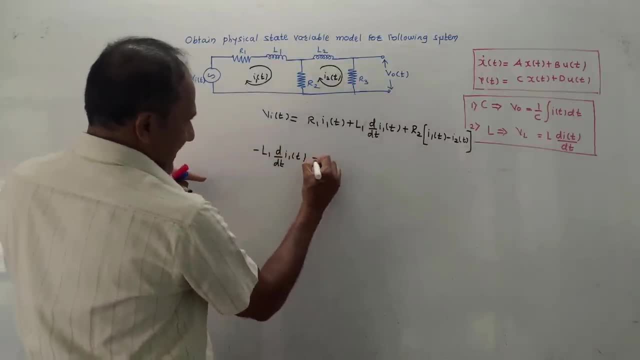 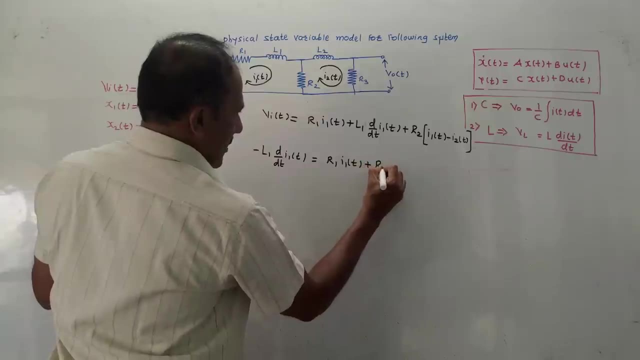 This term, d by dt term- I have transferred it at the LHS- is equal to this first term as it is R1- I1 of t. This term I have transferred Plus R2 in the bracket I1 of t, minus I2 of t. 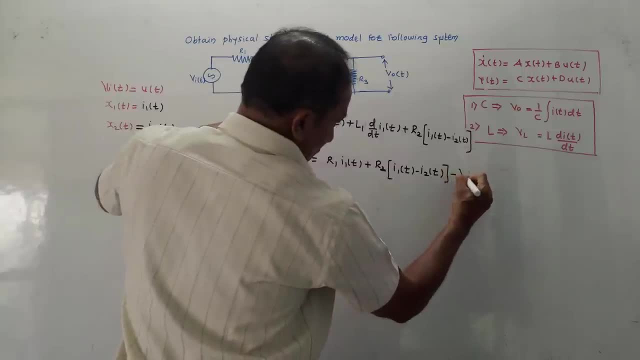 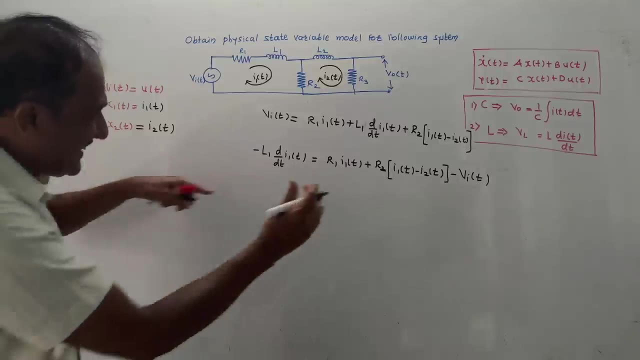 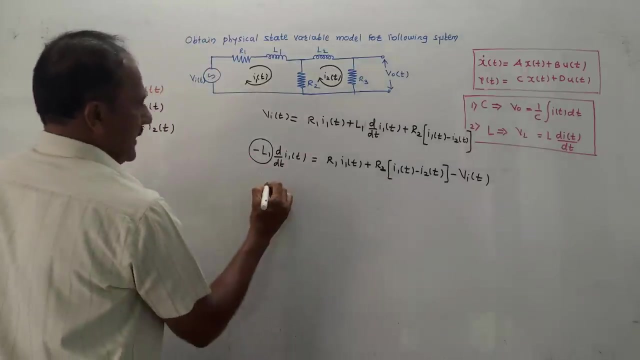 Now this term Vi of t, we will transfer it to RHS. So it becomes Minus Vi of t. But what is our rule? I want only d by dt of I1 of t at the LHS. So this term minus L1, I have to transfer it to RHS. 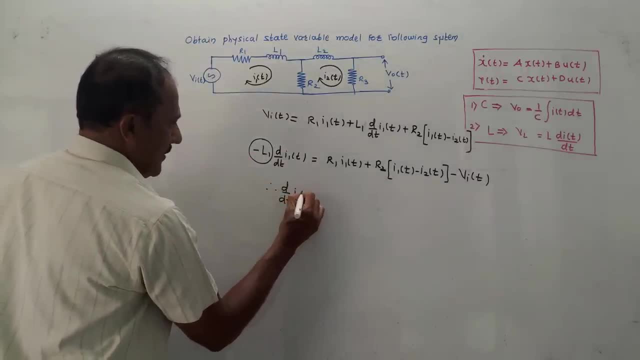 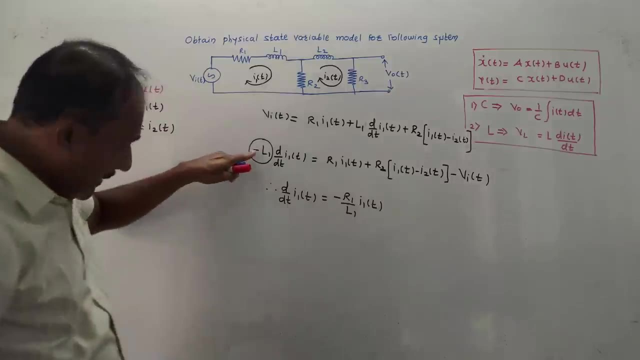 So I will write it like this: d by dt of I1 of t is equal to minus R1 upon L1 I1 of t. Keep in mind I am transferring this minus L1 to RHS. This becomes again minus R2 upon L1 I1 of t. 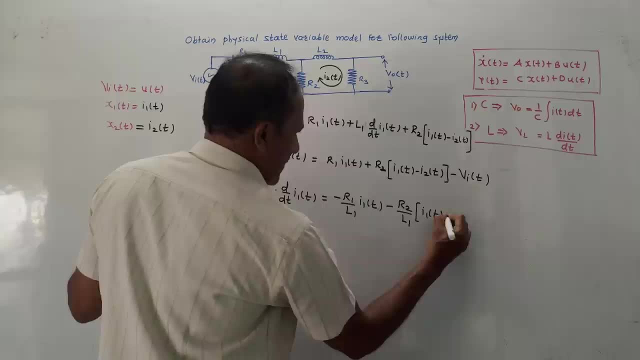 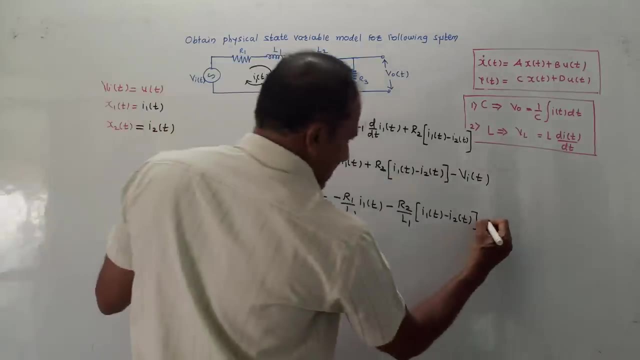 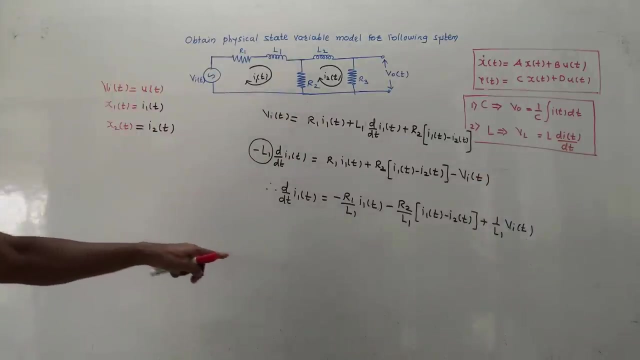 This becomes minus Minus R2 upon L1 in the bracket I1 of t minus I2 of t. This is already minus. This is again minus. Minus must become plus 1 by L1 Vi of t. Now I have to assign the notation which I have already. 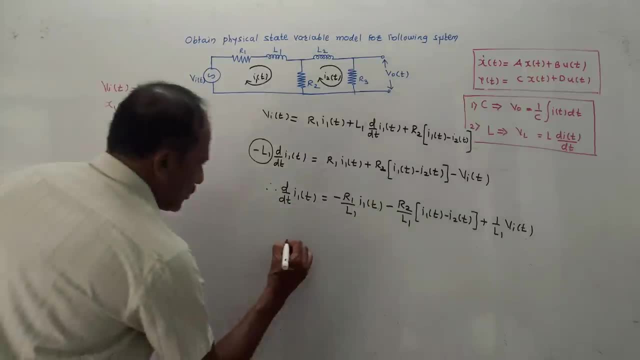 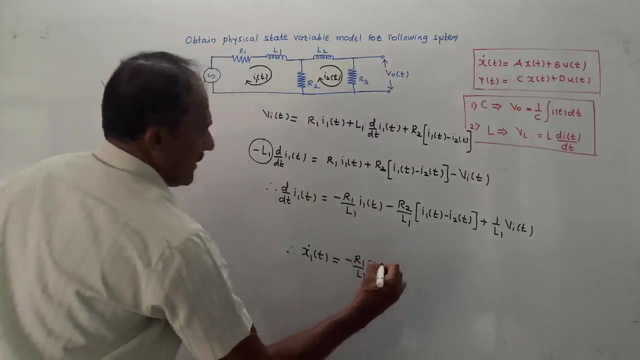 written So d by dt I1 of t. For I1 of t I have straight variable x1 of t, So I will write: X1. dot of t Is equal to I1 of t. equals to minus r1 upon l1. i1 of t is x1 of t, so it is x1 of t minus r2 by l1 in the bracket. 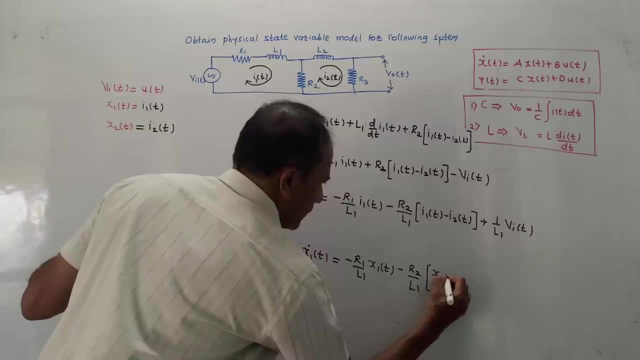 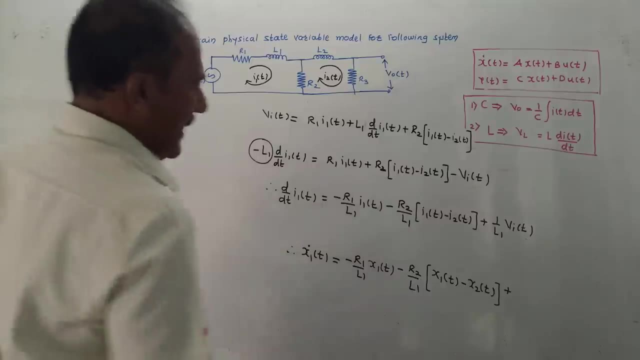 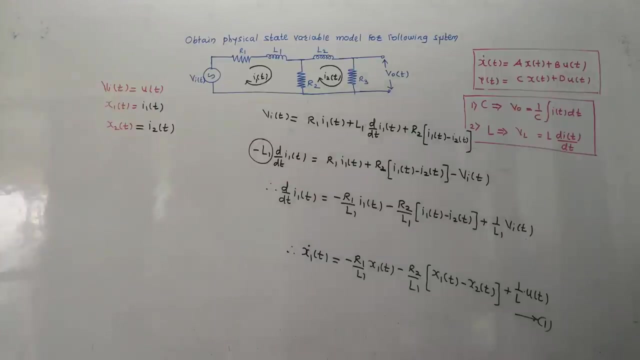 i1 of t is x1 of t, so it is x1 of t minus x2 of t plus 1 by l remains as it is x into u of t, say it is equation number 1. so i have prepared equation 1 related to the input. 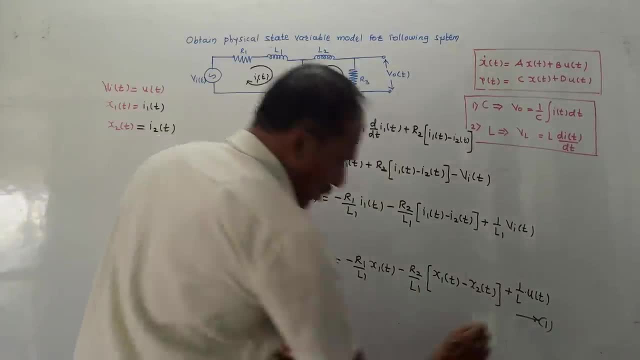 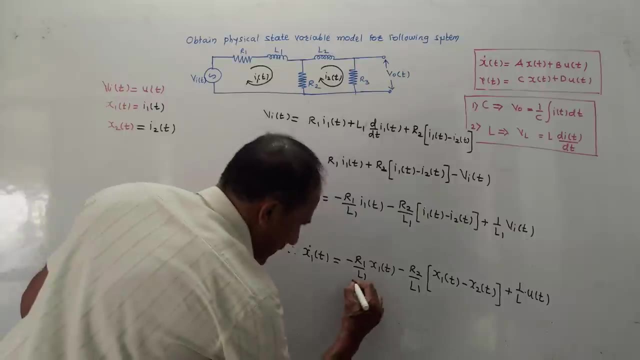 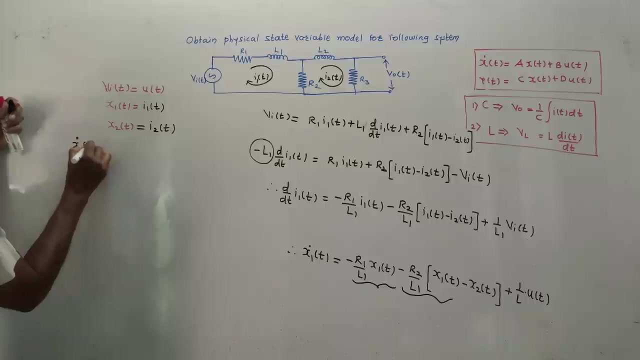 loop. now see, let us simplify it a little more. so i will just simplify it and then i will call it as equation number 1. x1 terms have to be collected means: look here, this term is of x1 and this is also of x1, so i will write it like this: x1 dot of t is equal to, as i told you. 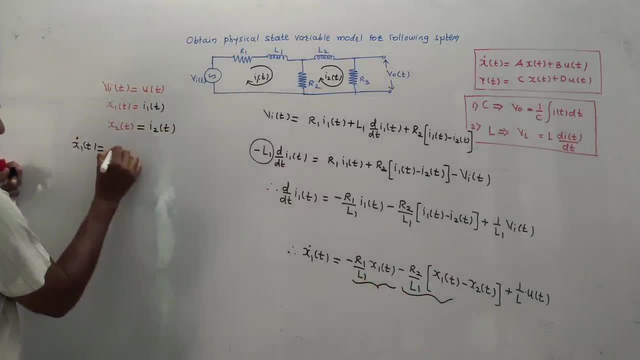 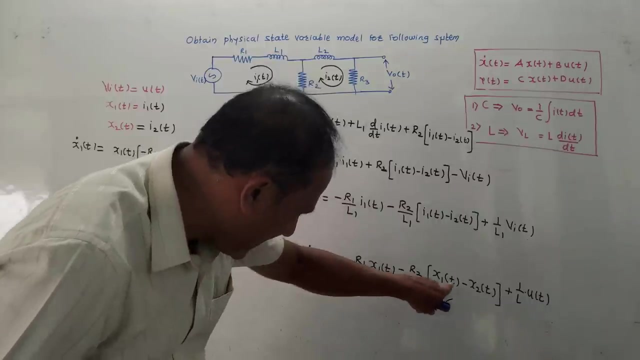 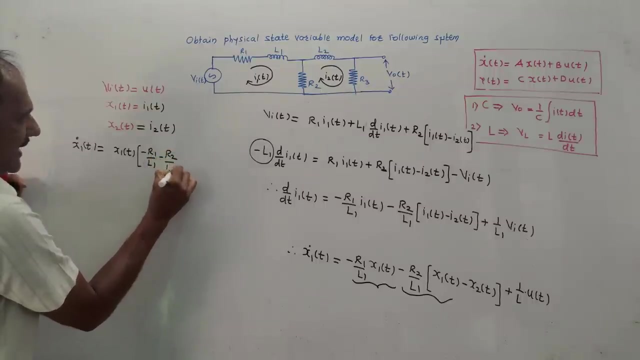 So I will write it like this: x1 of t in the bracket, minus r1 by l1,, minus r1 by l1, then this term will get multiplied with x1 of t, so it is minus r2 by l1.. 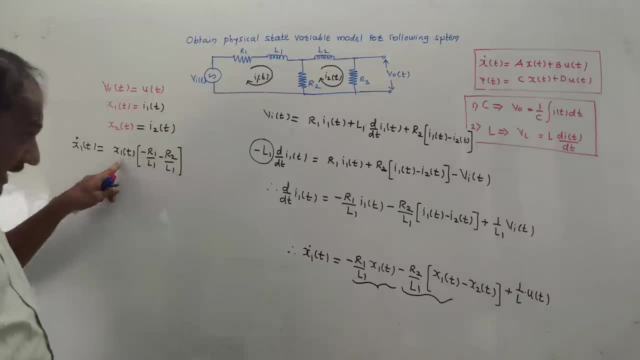 It is same as minus r1, minus r2 upon l1,. I have collected the terms of x1 of t. now see, this is not minus. we will multiply it inside. minus. minus becomes plus, so this term I can write it like this: r2 by l1, x2 of t plus 1 by l? u of t. this is equation number 1,. 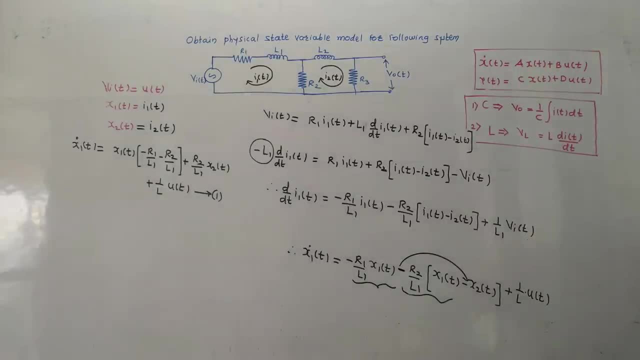 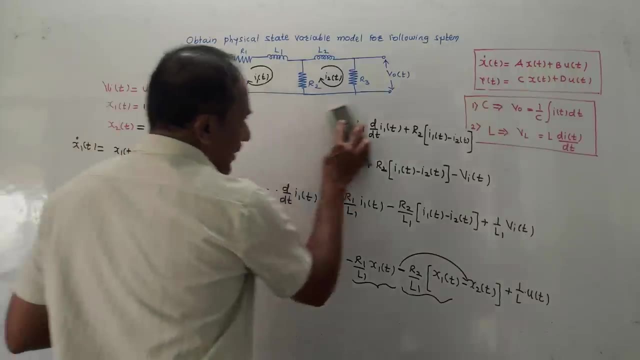 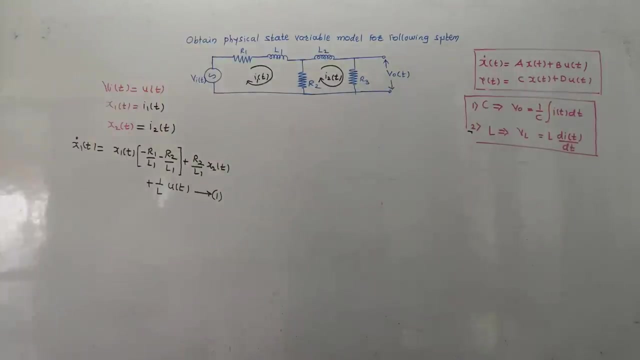 this equation is 1, related to the KVL which we have taken. So this is the same equation applied to loop 1.. Likewise, I will have to create one more equation related to KVL, which will be applied to loop 2.. 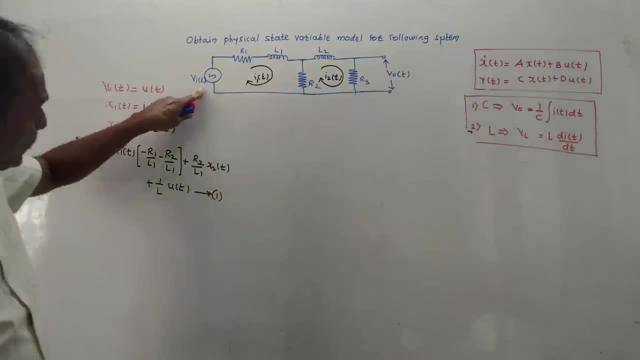 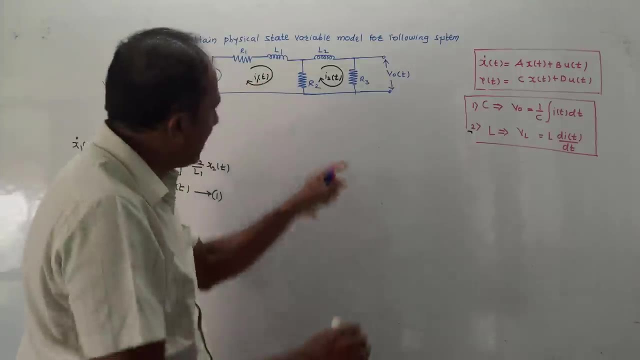 Now see we are using the same technique again. how we used the technique here. input voltage applied will be equal to voltage drop across all the elements which are in the first loop. same technique to be used. this is second loop. So voltage drop across all elements will be equal to applied voltage. but there is 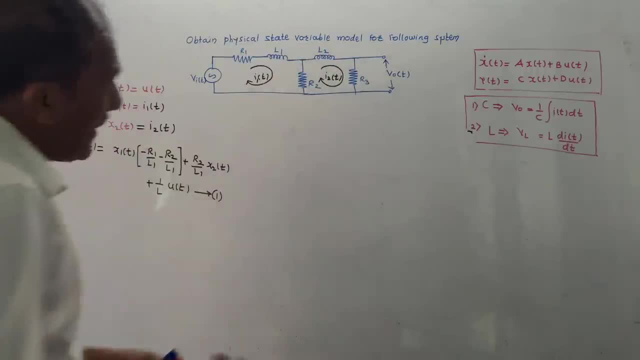 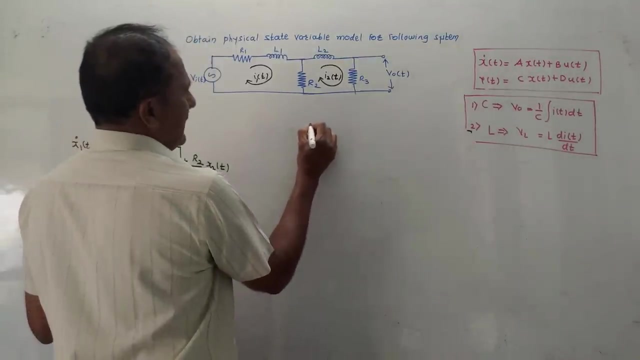 no applied voltage in the second loop. So while preparing the equation of output- I mean equation of KVL- for the second loop, I will consider applied voltage will be equal to 0. Means how to write the equation. since applied voltage is 0, I will write it like this: 0. 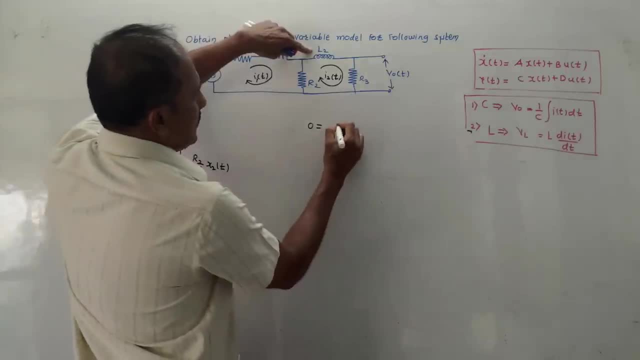 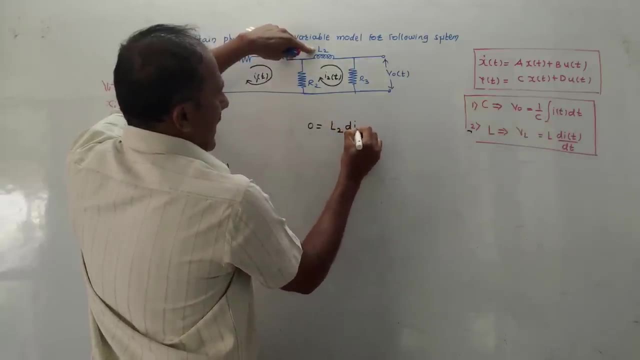 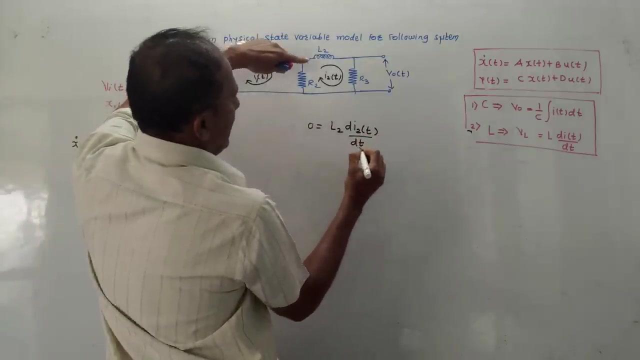 is equal to. I am talking about loop 2, let's start from here. suppose it is l2, so voltage across inductor is l2, di2t. So this is the first loop. See, I am talking about loop 2, so this current will be i2t, di2t by dt. 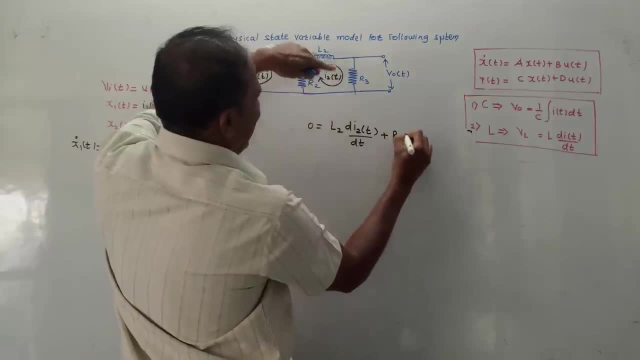 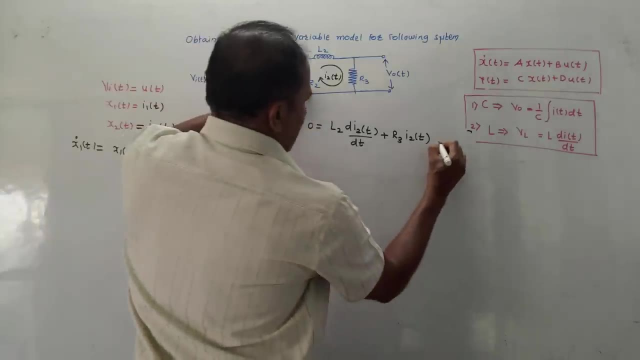 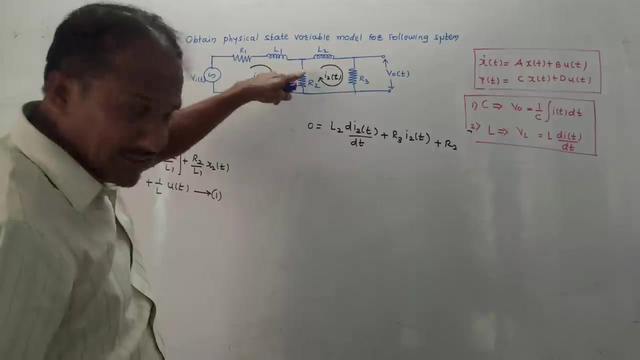 This is for inductor l2 plus R3 into i2 of t, R3 into i2 of t plus this is R2, so voltage drop across R2, here also we don't have to make a mistake- through R2 again, two currents. 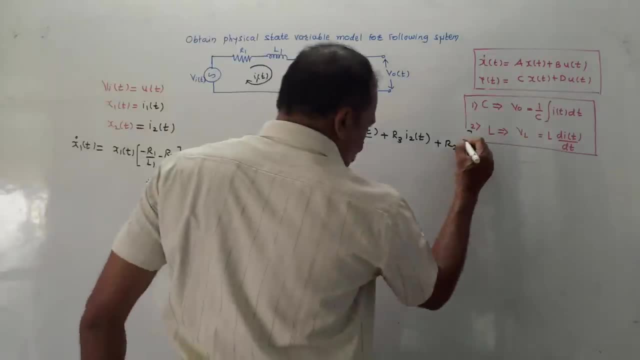 are flowing, but I am applying KVL for loop 2.. So for R2 we have to write i2t. So I am applying KVL for loop 2.. So I am applying KVL for loop 2.. 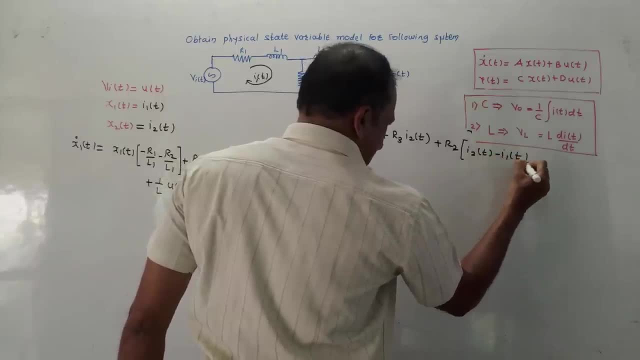 So I am applying KVL for loop 2.. So by applying this, I am not making a mistake. I am applying KVL for loop 3.. Now then we write KVL for loop 3.. So I am writing i2t minus i1 of t. 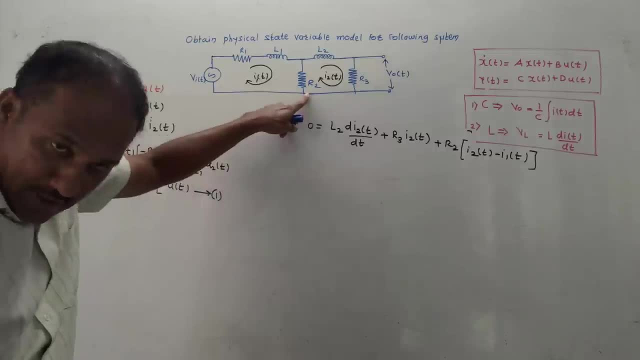 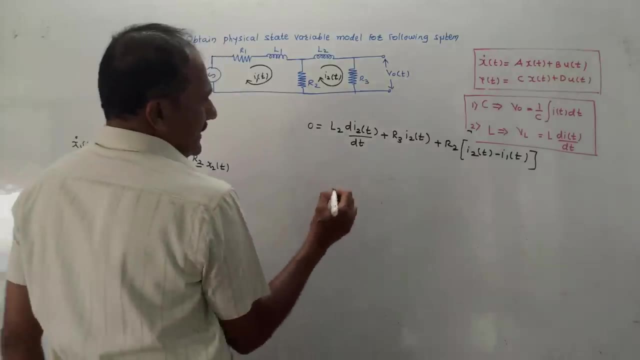 Here we have to avoid common mistakes. R2 is common, R3 is common for loop 1 and 2, but we are writing a equation for loop 2, so it will be i2 minus i1, like this. Now let us simplify it. we know the rule. 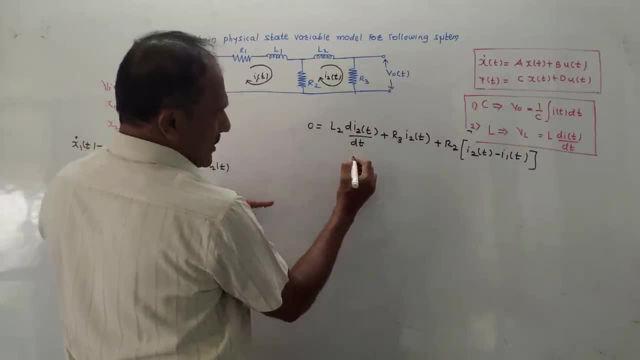 This whole term. first rearrange and write like this: 0 is equal to l2 di2t by dt plus R3 into i2 of t plus R3 i2 of t. so this will be i1 minus i2 of t. 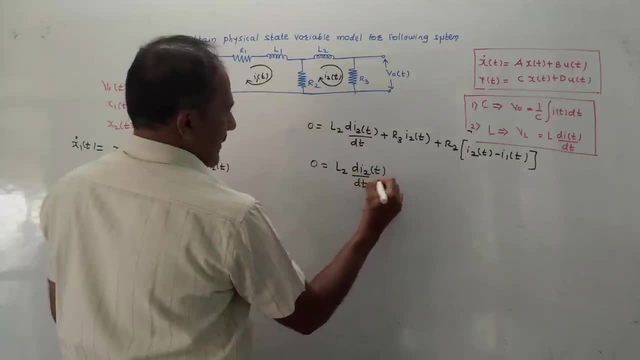 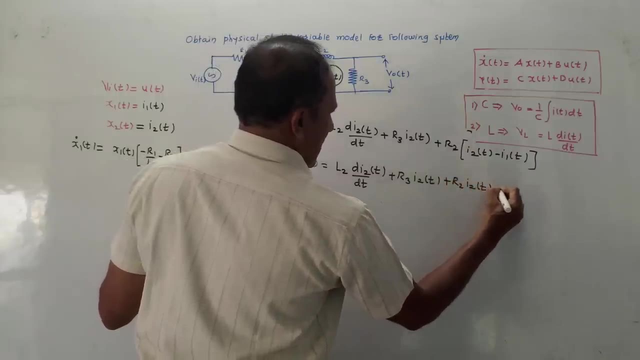 So I am writing the equation for loop 1 and 2, like this: I2T by DT plus R3, I2 of T plus R2, I2 of T minus R2, I1 of T. I have already simplified this. 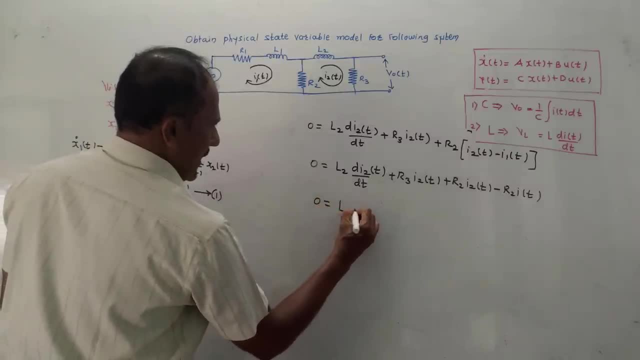 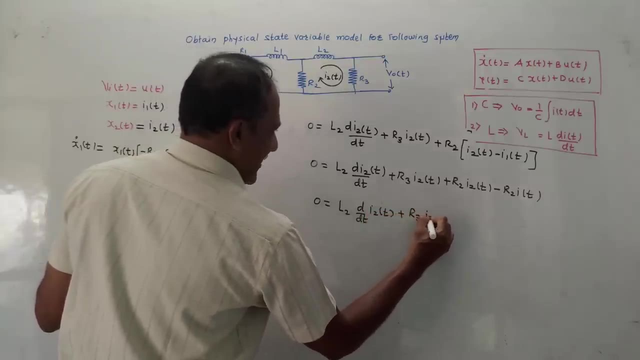 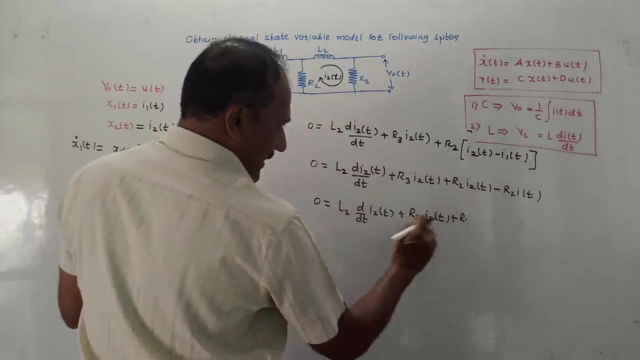 So I will write it like this: 0 is equal to L2 D by DT of I2 of T plus R3- I2 of T plus R2.. Now see R2- I2 of T or R3- I2 of T. these two terms can be combined and this is I1 of T. 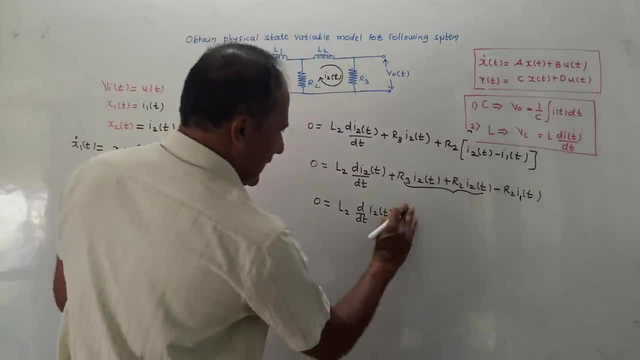 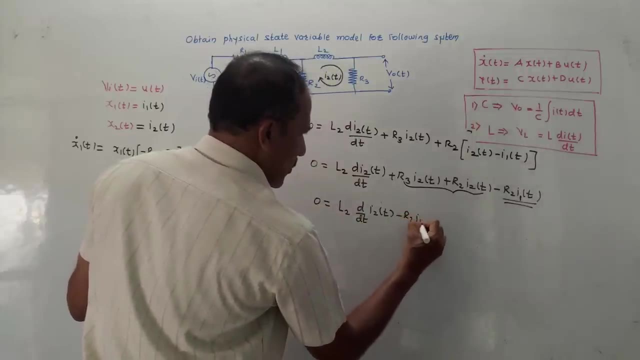 So I will rearrange it like this: First let's write the term I1 of T Means. first I will write this term minus, this term minus R2 into I1 of T plus. With this we can take I2 of T as common. 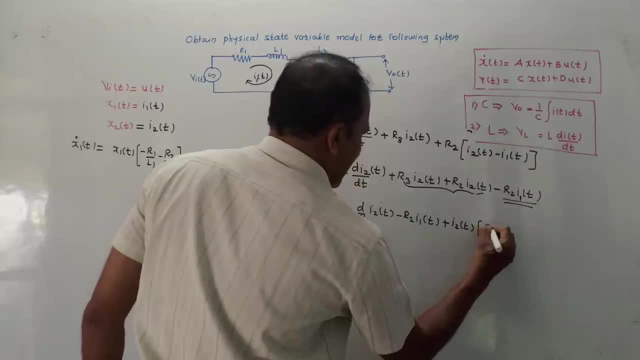 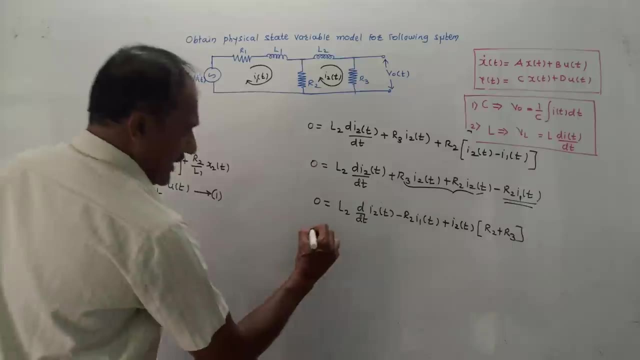 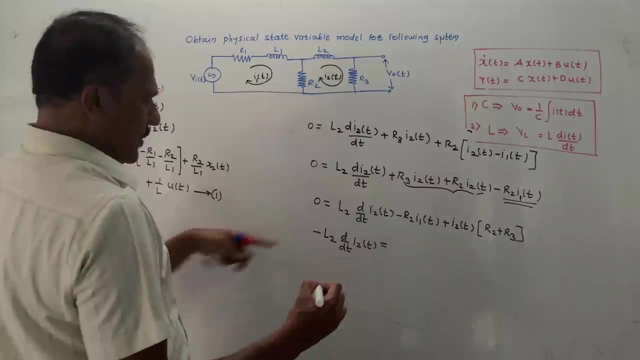 So I2 of T in the bracket R2 plus R3.. Now, as usual, D by DT term is in LHS, So it becomes minus L2. D by DT of I2 of T will be equals to. Remaining terms are as it is. 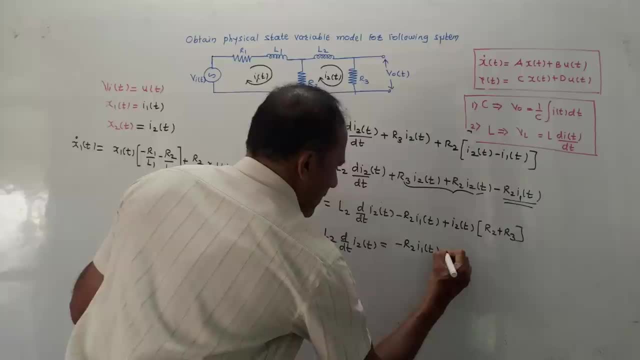 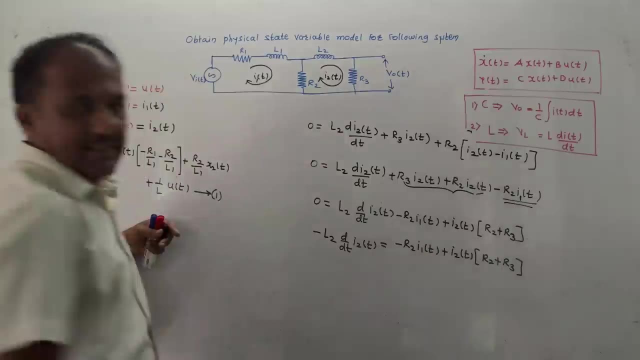 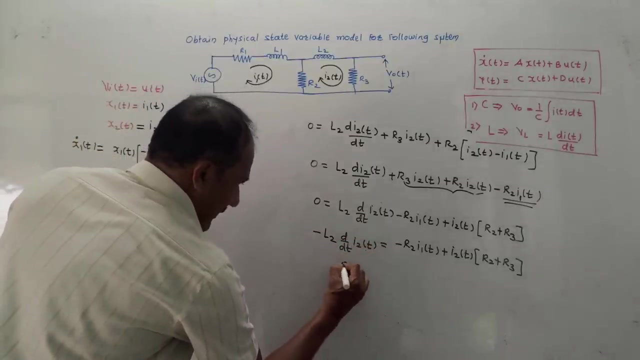 Minus R2: I1 of T plus I2 of T in the bracket R2 plus R3.. It is R2 plus R3.. Now I want only D by DT of I2 of T at the LHS. So we will transfer this. 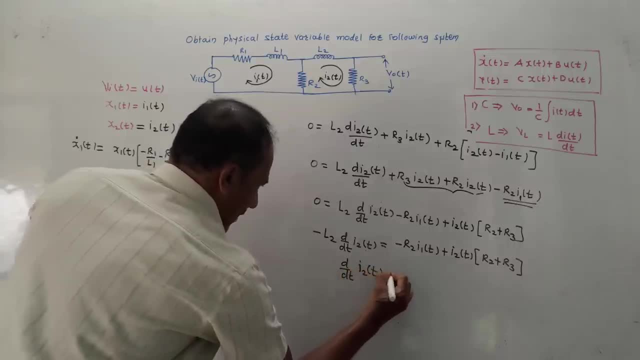 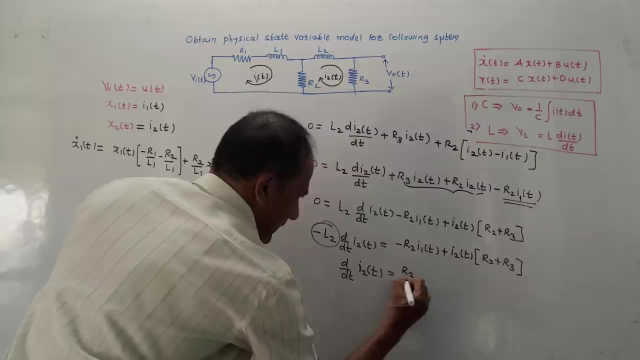 Here I will write D by DT of I2 of T. I will transfer this minus L2 at the LHS. I am transferring this minus L2 at the LHS So it becomes plus R2 by L2. I1 of T minus. 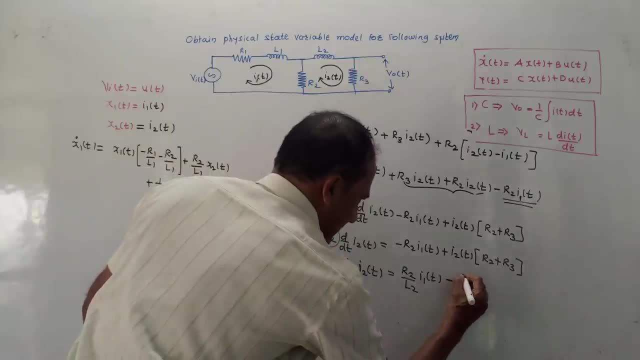 See, I am transferring this L2 here, So I will write it like this: Minus R2, plus R3 upon L2.. Into I2 of T: One and the same thing. Now we have to use variables, So we know the rule. 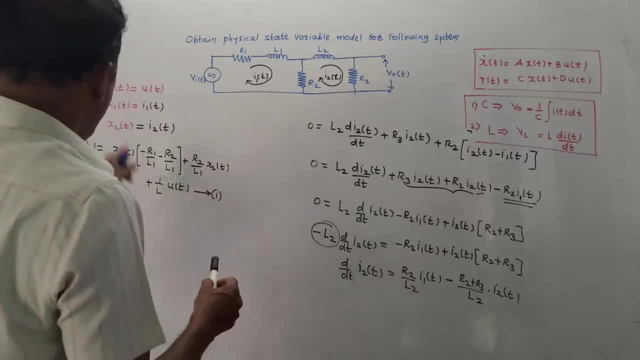 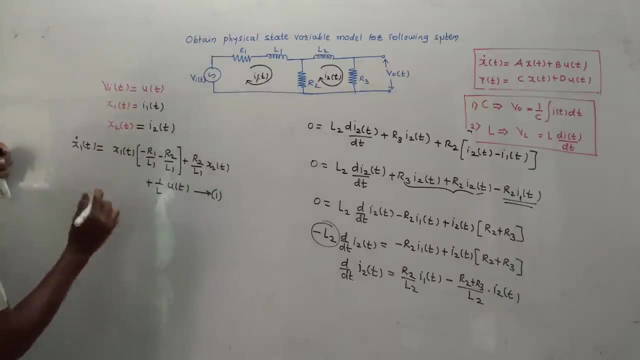 We will use variables, So D by DT of I2 of T. For I2 of T the variable is X2 of T. So here I will write this equation: So D by DT of I2 of T, I2 of T means X2 of T. 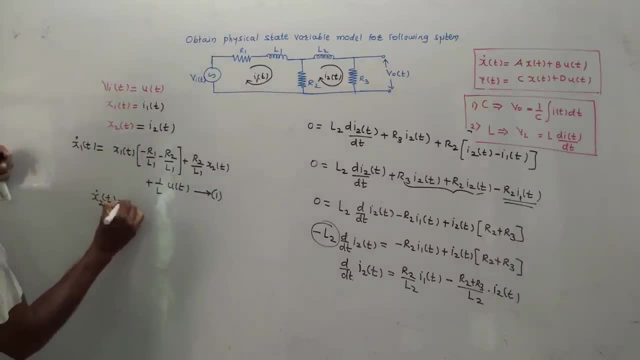 So it becomes X2. dot of T is equals to. We know the rule D by DT means dot mark. I2 of T means X2 of T is equals to R2 by R3.. L2 into I1 of T. 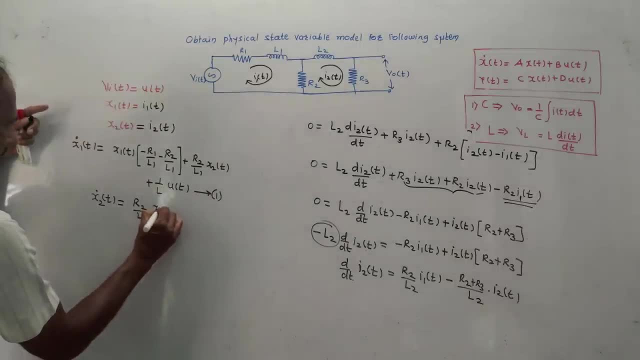 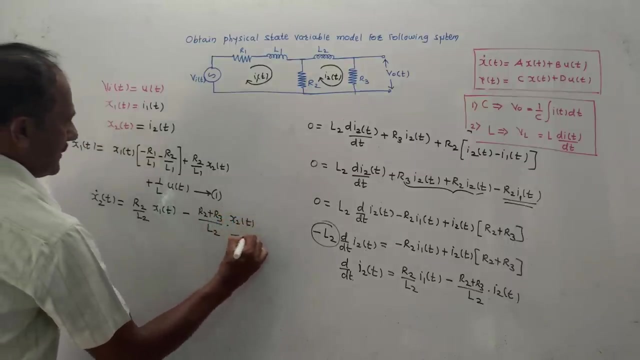 I1 of T's variable is X1 of T, So it is X1 of T Minus this term R2 plus R3 upon L2 into I2 of T. I2 of T means X2 of T. This is equation number 2.. 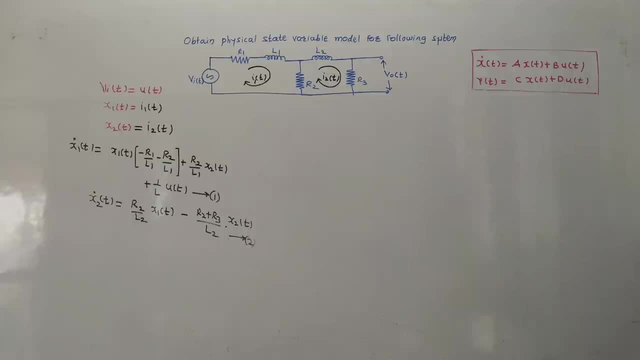 Which I got by applying KVL for loop 2.. Now let us write the equation of output also. So output. I write the equation of output here. Output is Y of T, is equals to V0 of T, Which is equals to voltage drop across R3 of T. 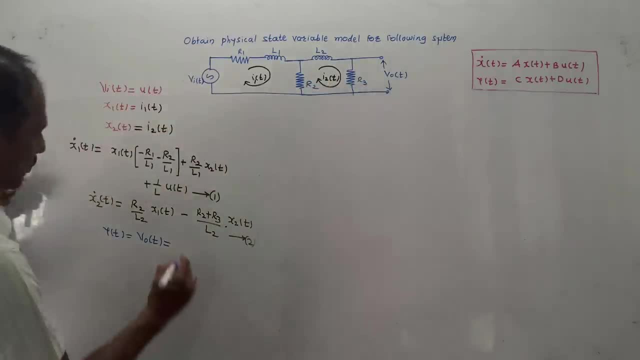 And through R3 of T, current I2 of T is flowing, So it becomes I2 of 2 into R3.. Therefore, in terms of notation I will write it like this: Which is equals to I2 of T. 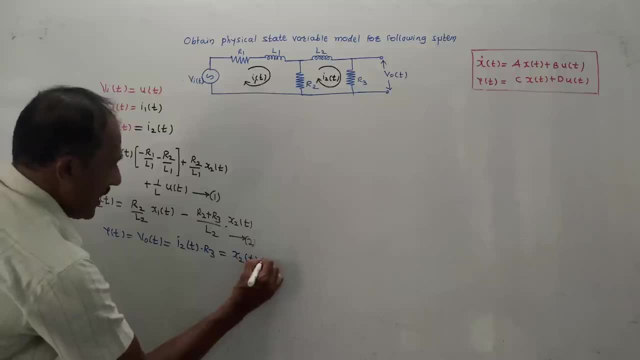 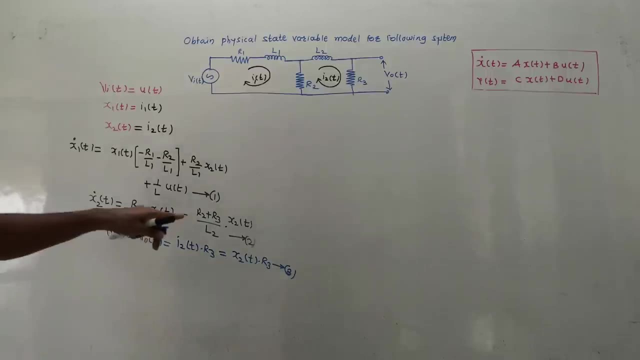 This is equation number 2.. Now, by making use of these equations, I will have to write the state model in terms of matrix, like the previous case. So we have to use this formula. X dot of T Means this equation. 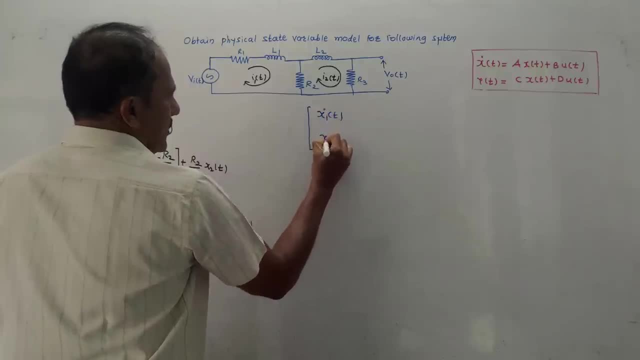 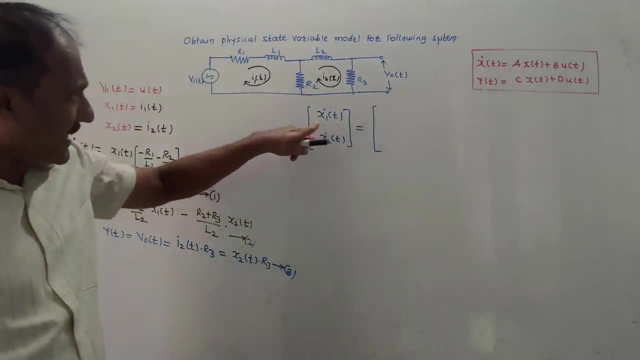 First in LHS I write X1 dot of T. Second term will be X2 dot of T. Then matrix A, First row. First row is related to equation number 1.. That is equation of X1 dot of T. 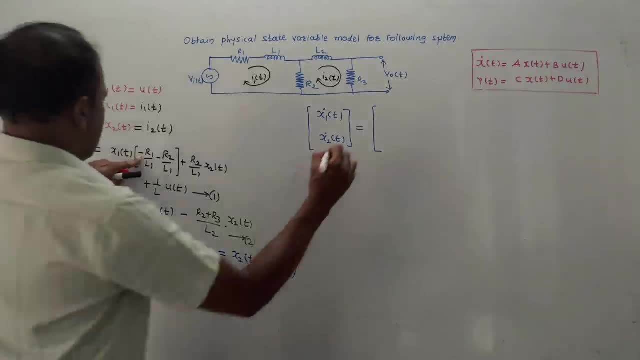 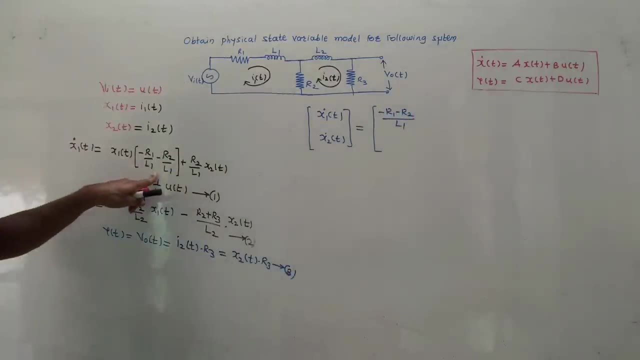 This is equation number 1.. First look at the coefficient here. This is minus R1, minus R2 upon L1.. We can take L1 as common in both, So I have written it like this: This is the coefficient of X1.. 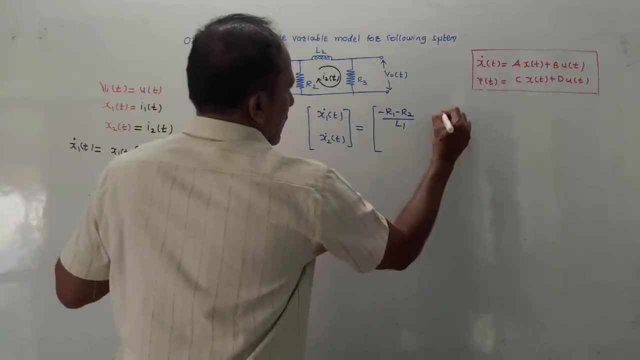 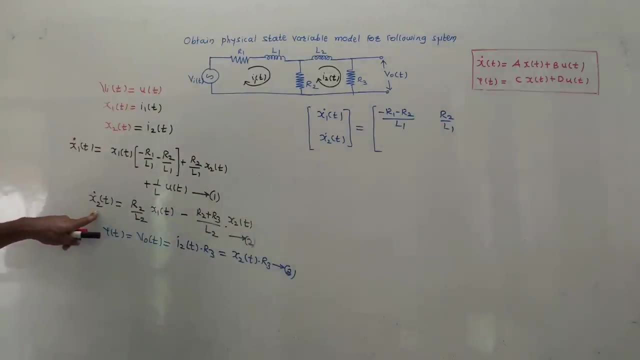 Coefficient of X2 is R2 by L1.. So this will be R2 by L1.. Now second row. Second row. For this I need to refer equation of X2, dot of T, That is, equation number 2.. 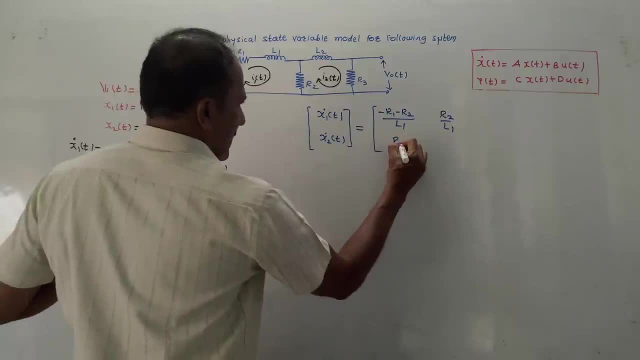 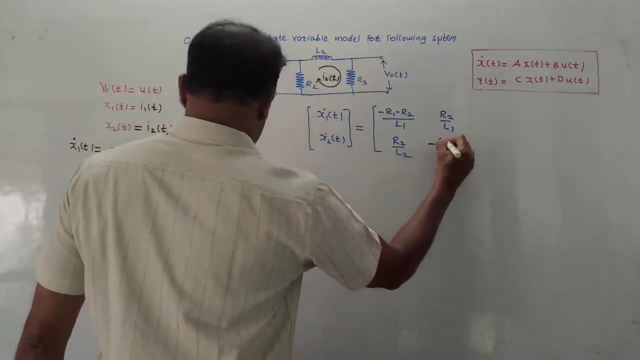 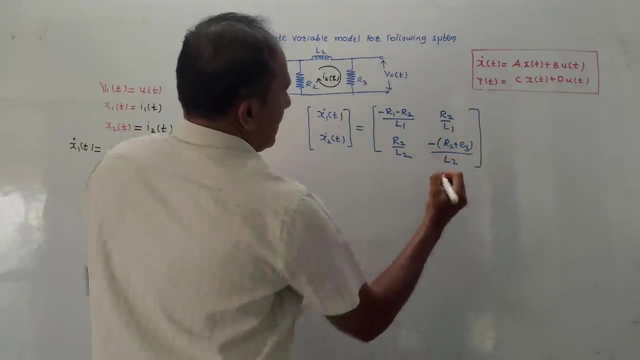 First coefficient is R2 upon L2.. So it is R2 upon L2.. Second coefficient: This coefficient Minus- I will write it like this- Minus R2 plus R3 upon L2.. This is the matrix A. 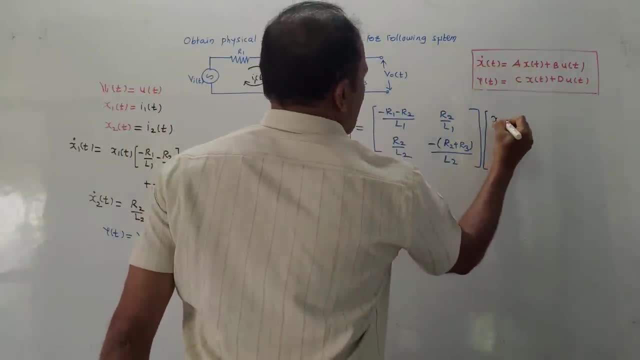 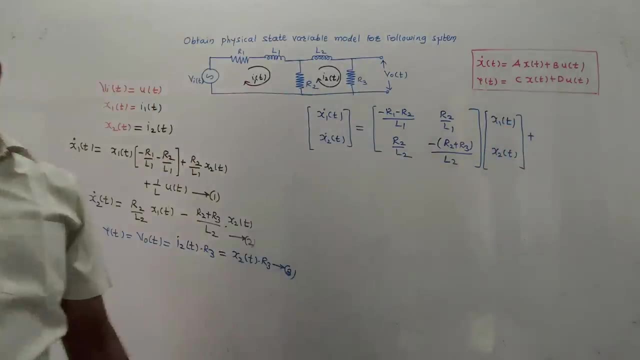 Into X of T. Here I will write X1 of T. Here I will write X2 of T Plus B into U of T. Now look In equation 1, U of T. There is no U of T term in equation 2.. 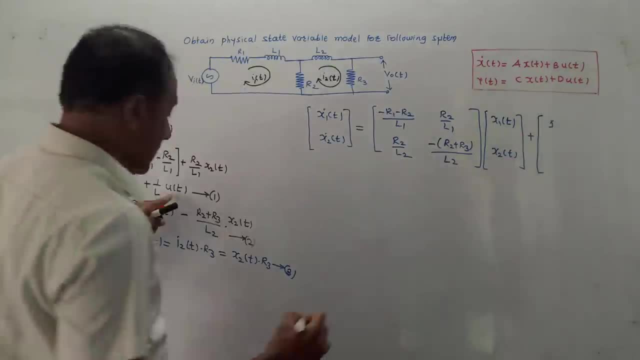 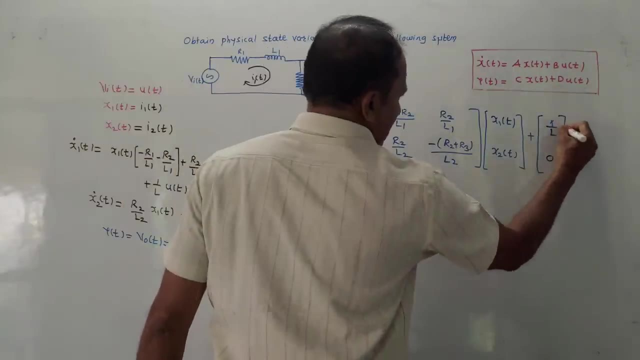 So I will write it like this: 1 because this is 1 by L, So it is 1 by L. 1 by L into U of T, So it is 1 by L. Second term is 0 into U of T. 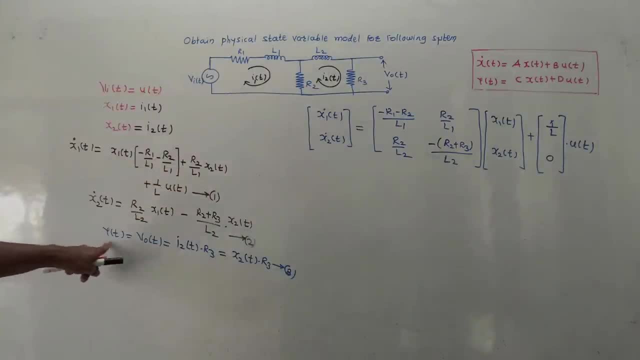 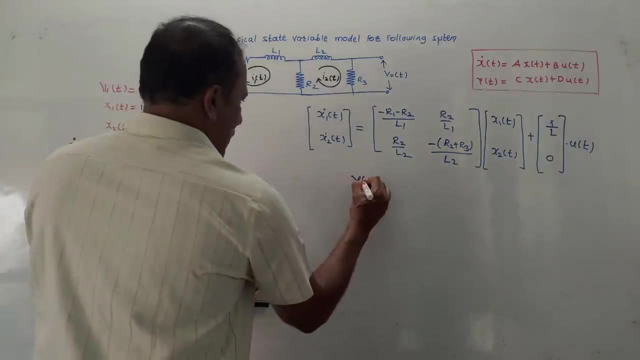 Now for the second model, second matrix. I will have to refer equation of output. It is very simple. It is X2 of T into R3.. There is no X1 of T term, So I will write it like this: 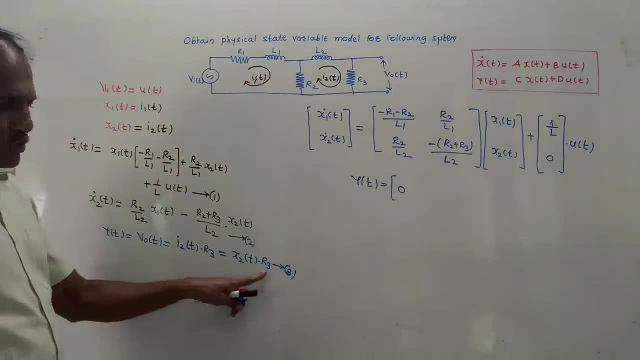 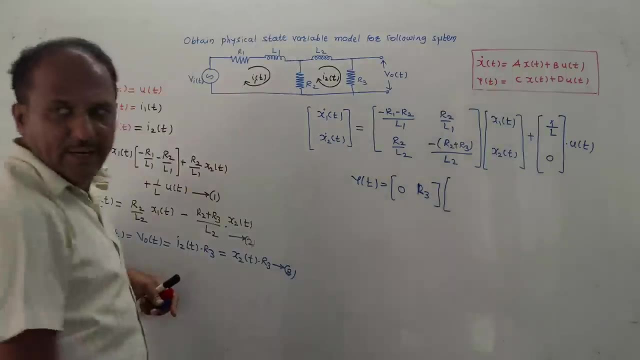 No X1 of T term is there, So it is 0.. Coefficient of X2 of T is R3.. So it is R3.. This is R3.. Here I will be writing X1 and X2 as a column matrix. 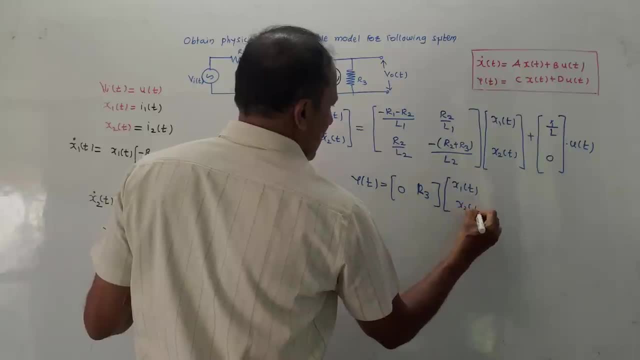 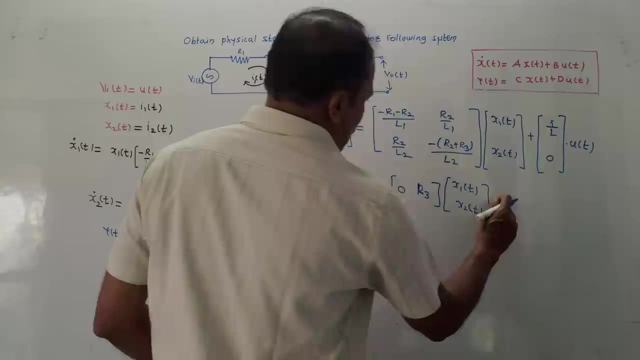 So it is X1 of T, X2 of T Plus. there is no U of T related to equation number 3.. That is equation of output. So that is optional. You may write 0 U of T, Alright. 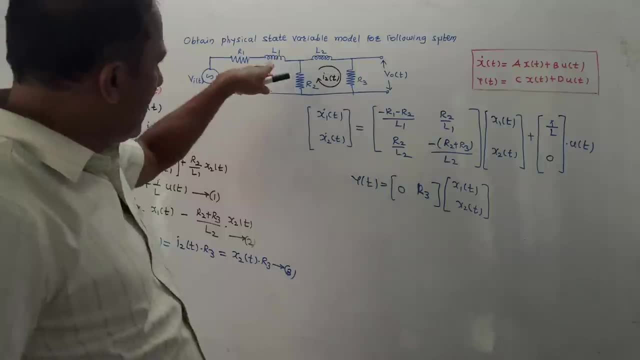 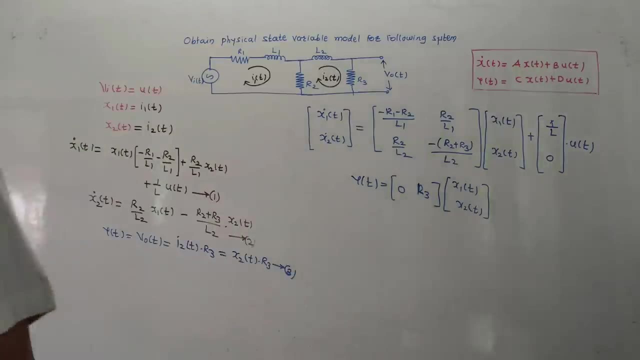 So this is about the state model of the given diagram, given system. So, dear students, that's it for today's session. So thank you, Thanks a lot for watching. Thanks for watching this video.